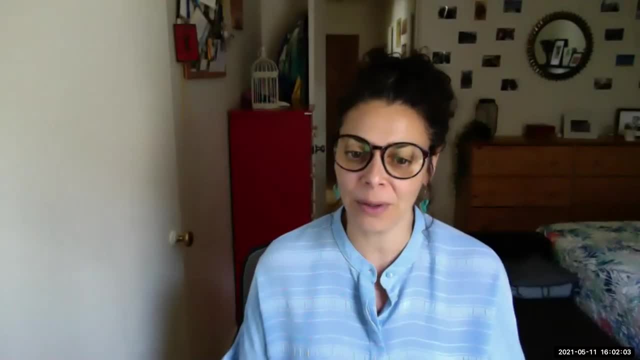 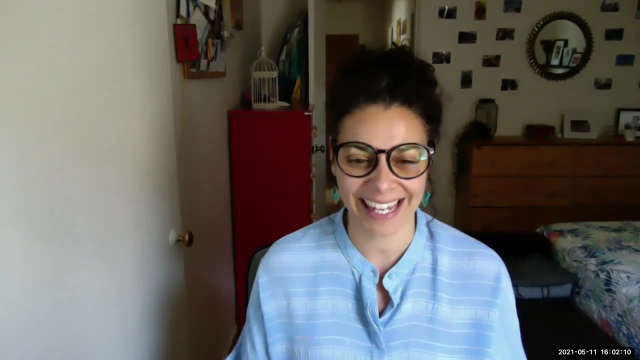 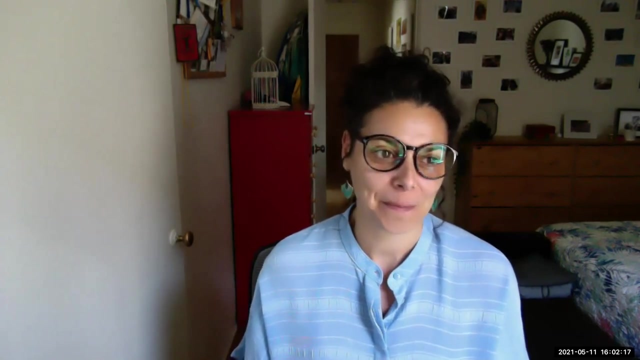 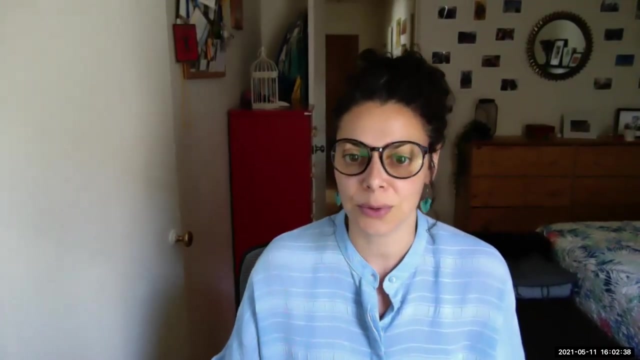 Okay, Hello everyone. I can see people is connecting, So very nice to Hey Hannah, Hey Cindy, So many known faces. We're going to give like two more minutes for people to connect and we will start And people can choose to keep their cameras working or not working. Feel free to choose. 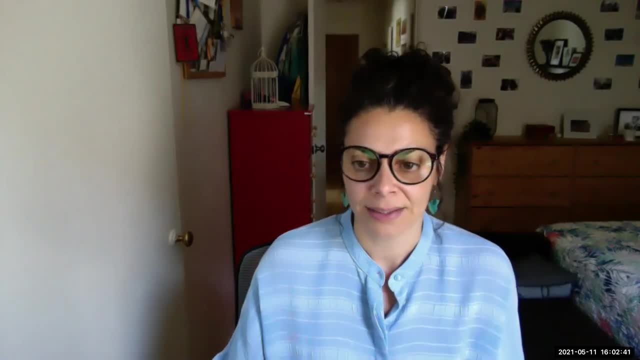 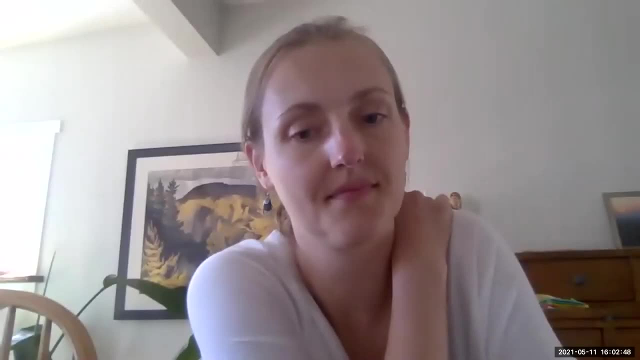 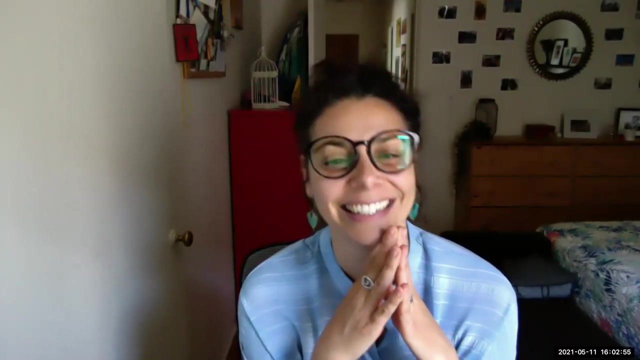 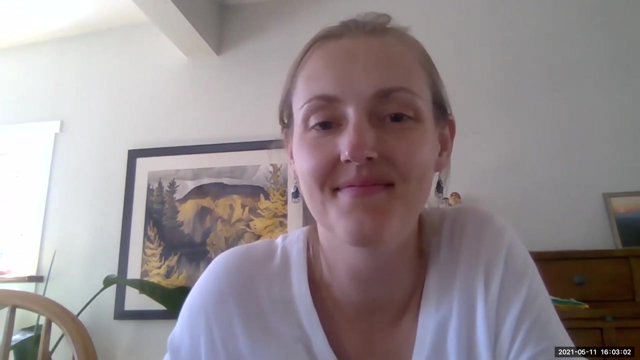 whatever you feel more comfortable with. I hope everyone- everyone who is in Vancouver, I'm sure- is enjoying this glorious sunny day. We have been very lucky. Yeah, So I think I can. Okay, I see 15 participants, but I want to make sure that 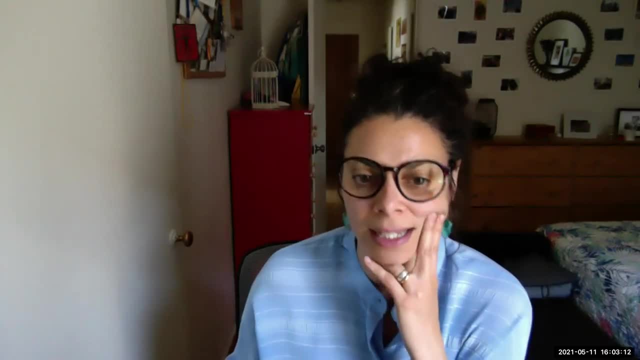 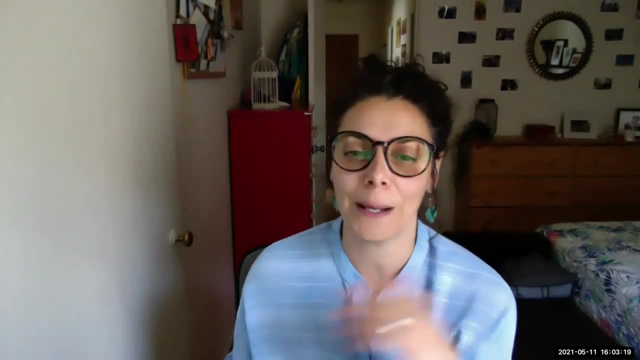 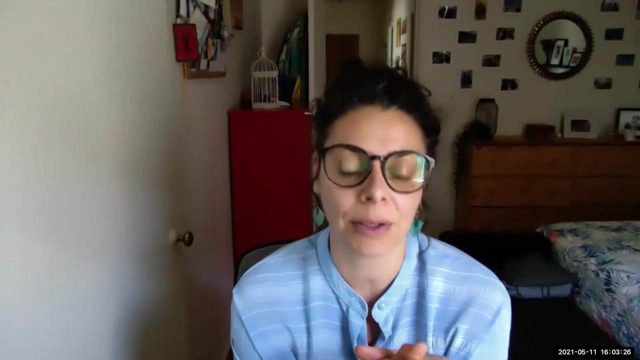 we have time for questions, So I think I'm going to start introducing myself and just basically introducing the seminar. So welcome everyone And thank you for joining us for this month. CSFS Associate Seminars. My name is Laura Morillas and I am the Research Manager. 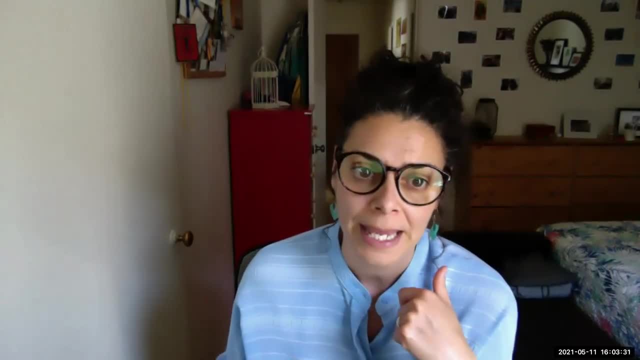 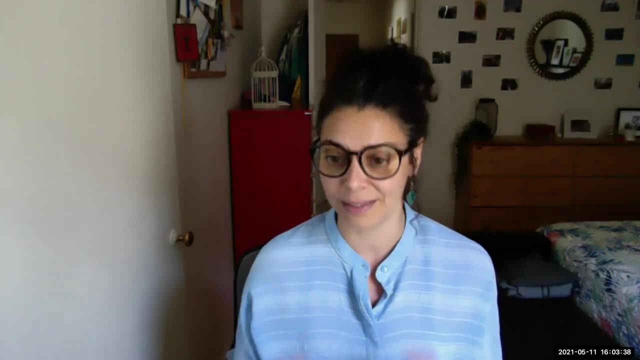 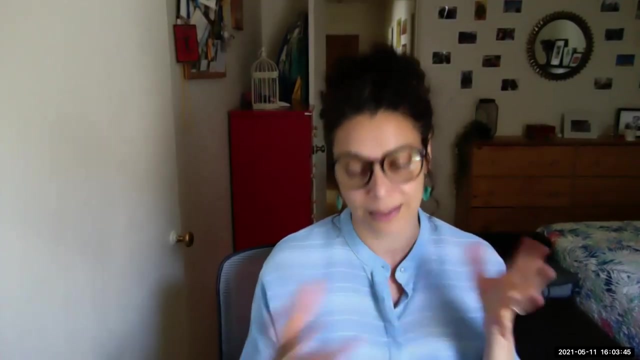 at the Center for Sustainable Food Systems, And I'm also the Director of the Center for Sustainable Food Systems at UBC Farm. And first of all, I would like to begin acknowledging that UBC, the university that we are, most of us, part of, it's located in Vancouver campus. Well, the Vancouver campus of UBC, the one, 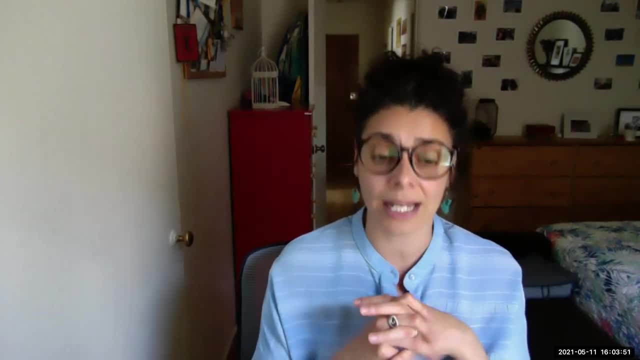 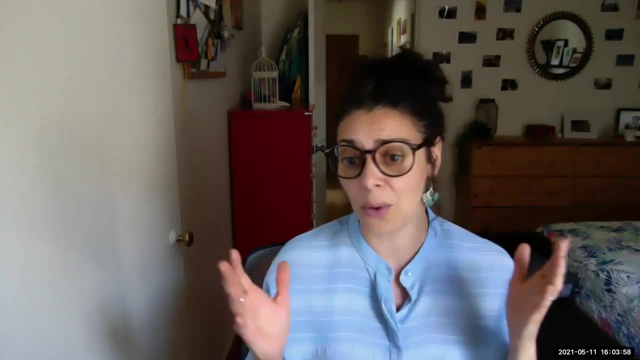 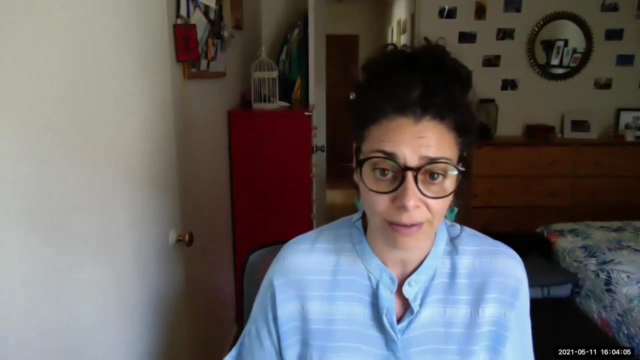 in Okanagan is situated on the traditional, ancestral, un-unceded territory of the Musqueam people, And I also know that right now that we are in this virtual world, many of you might be joining this meeting from other places near and far, And I would also like to invite you to acknowledge and to consider and have 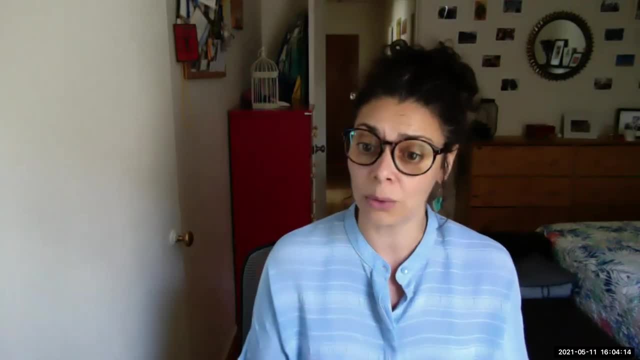 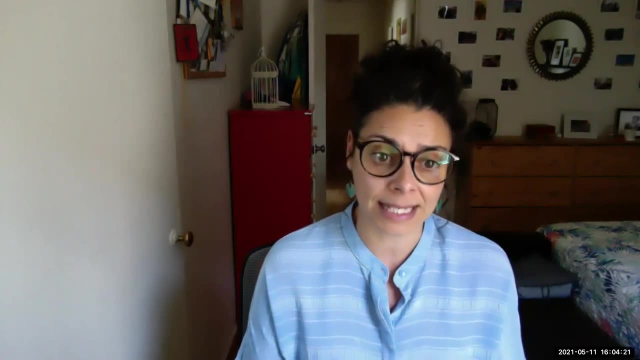 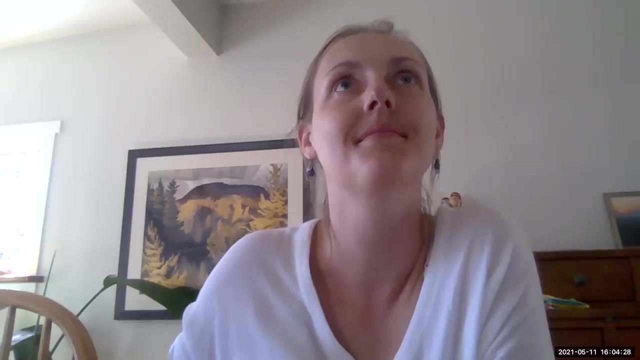 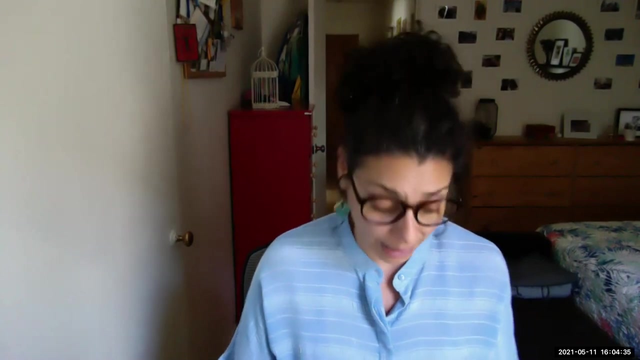 a minute to think about who are the caretakers of those lands, where you are right now and where you reside, And basically ask yourself: how are you accountable to those people, the people of those lands? And if you don't know what territories you are on, I'd like to encourage people to find 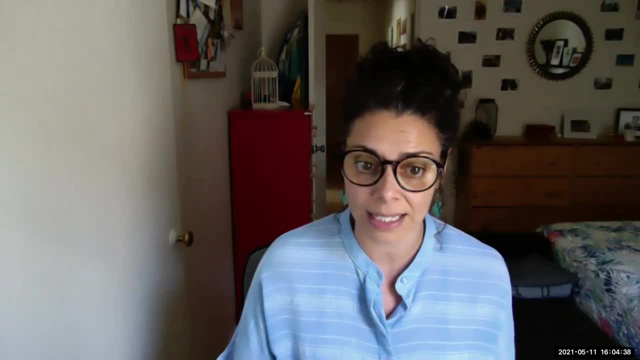 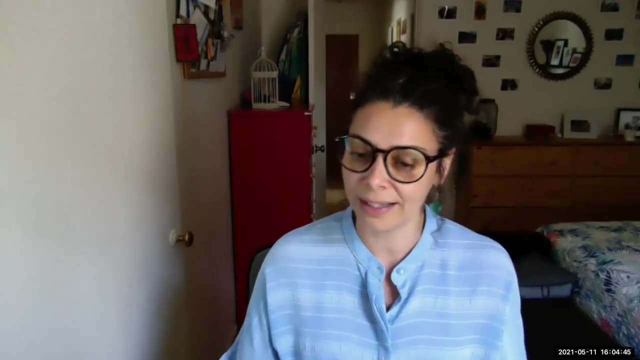 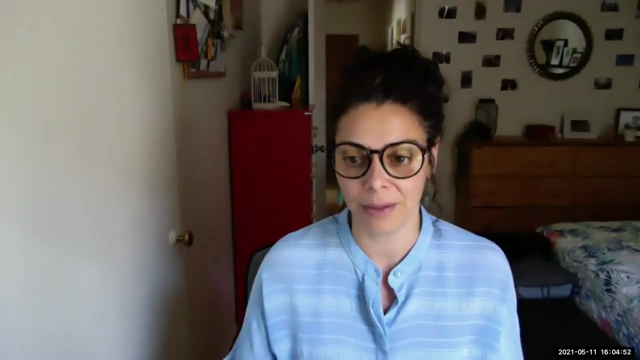 out, do a little bit of research. I am adding right now in the chat a resource that everyone can use to find out what are the traditional caretakers of those lands. Yeah, and I personally feel very grateful and very privileged to live and experience now my life in the Musqueam. 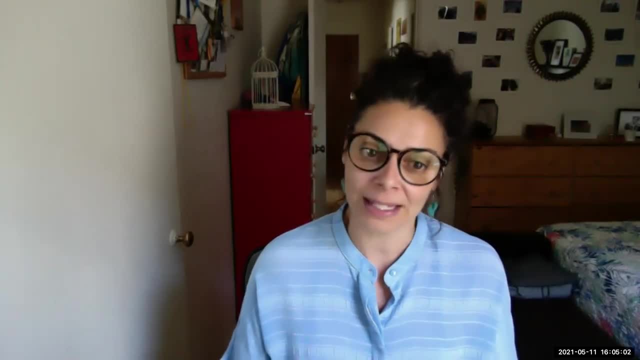 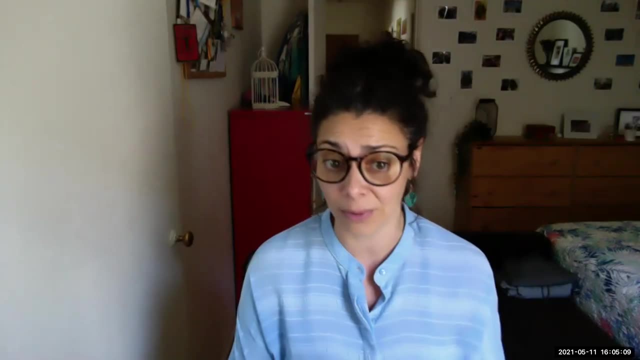 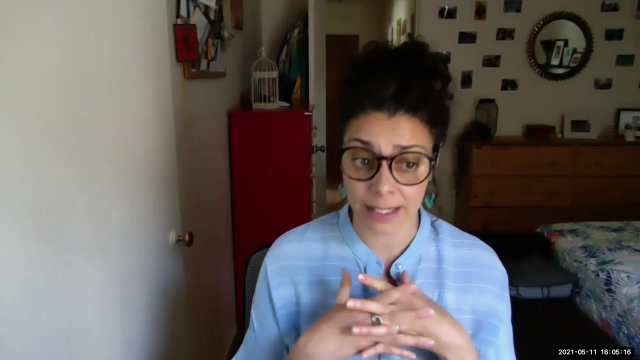 people lands. That's the first thing I always like to start with. And other than that, well this, welcome everyone. this seminar is organized by the Center for Sustainable Food Systems at UBC Farm. The Center is a teaching and research center as well as a local to global. 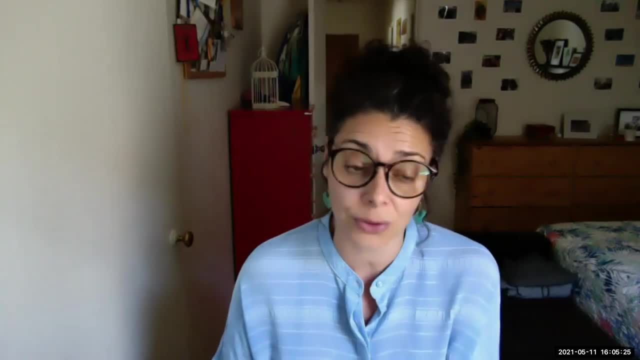 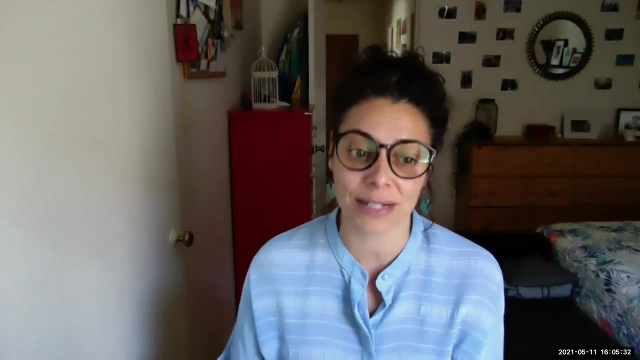 food hub, working towards a more sustainable food secure future. Our mission is to innovate, to be a global food hub and to be a sustainable food secure future. And our mission is to, from the field to the fork, to achieve a resilient, thriving and socially just food systems for all. 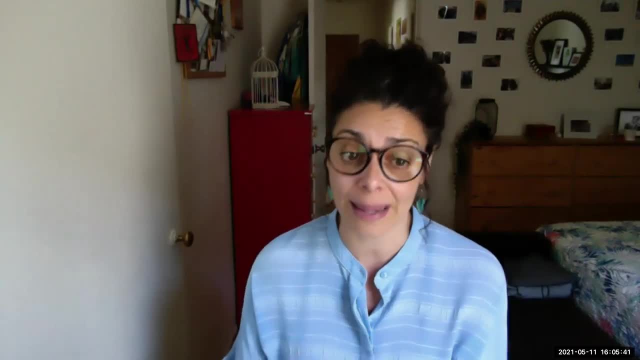 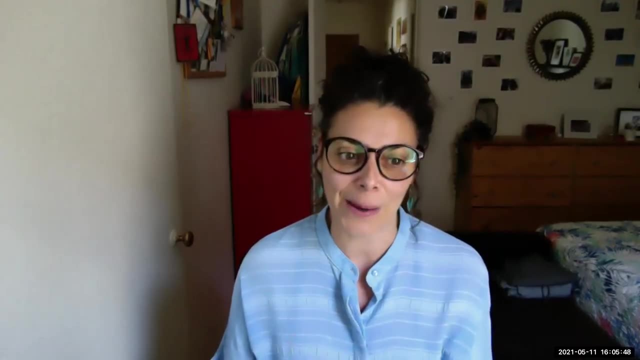 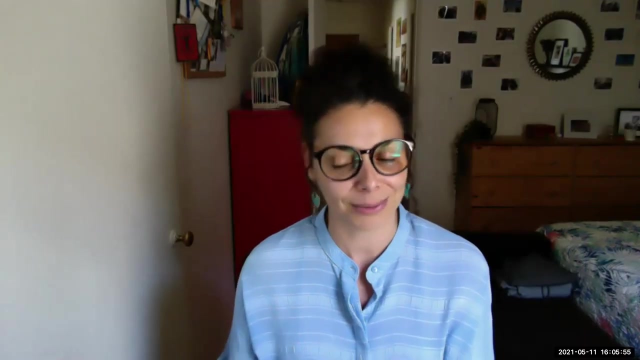 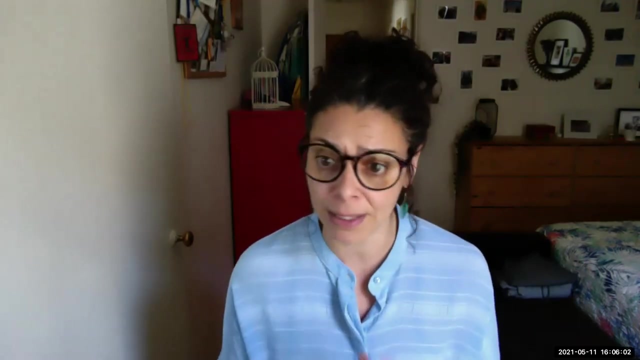 And today's seminar topic is adaptation and mitigation- dual objectives for addressing climate change in diversified agricultural systems- and our wonderful speaker, Dr Kira Borden, will tell us everything about that, or like the parts that she knows of and the parts that she's working on, And first of all, just a little bit of housekeeping. this is a. this is a meeting, so 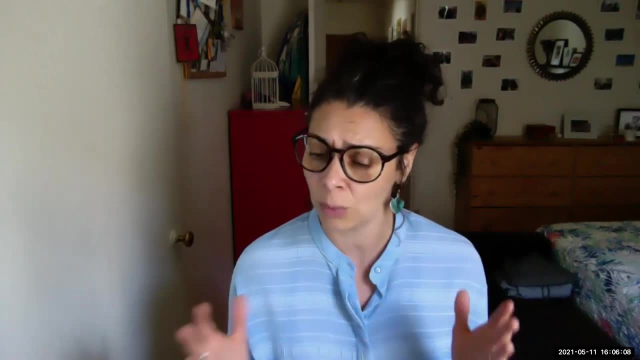 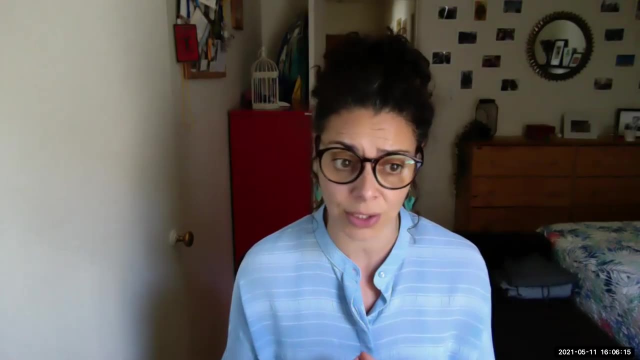 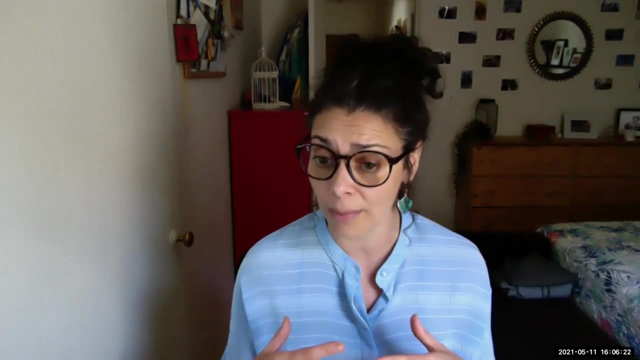 actually once we have like. we estimate that the presentation is going to be around 40 minutes and then we will have 15 minutes for a Q&A section, and so as questions arise during the presentation, you can add those questions in the comments in the chat, but at the end of the presentation 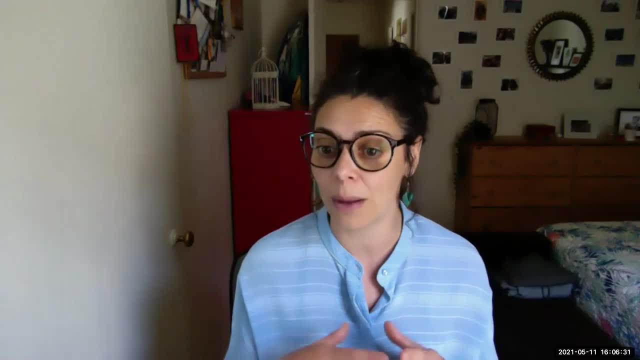 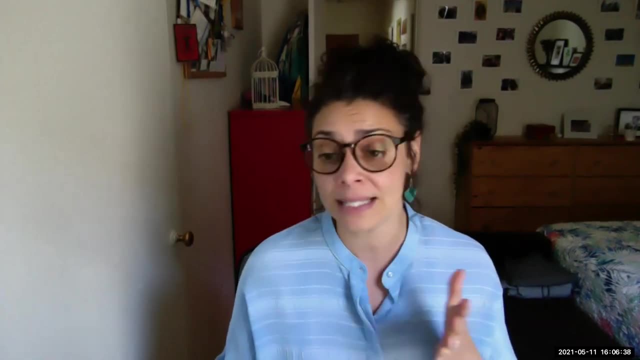 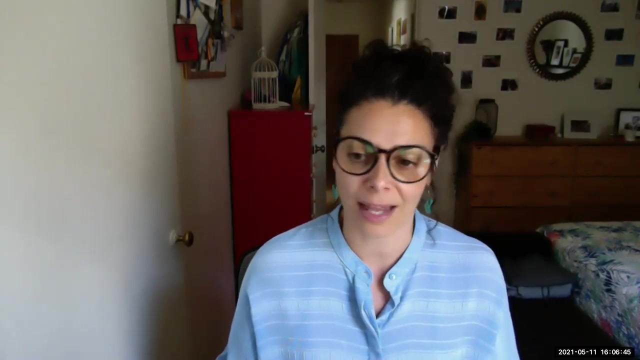 in the Q&A session, I most likely will ask you to unmute yourself and ask your own questions, because that's nicer, Yeah, and that's all. please keep up like. mute your microphones during the presentation so Kira doesn't suffer any sounds, and yeah, and with all that, it's my pleasure. 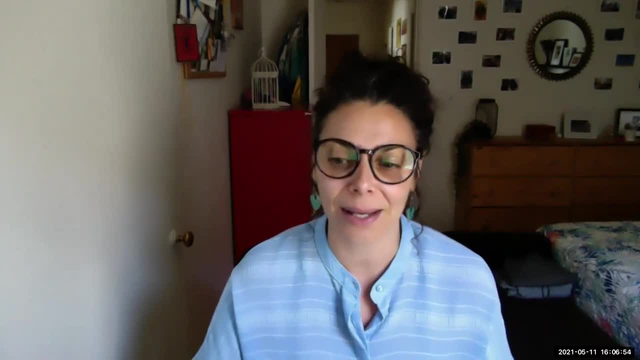 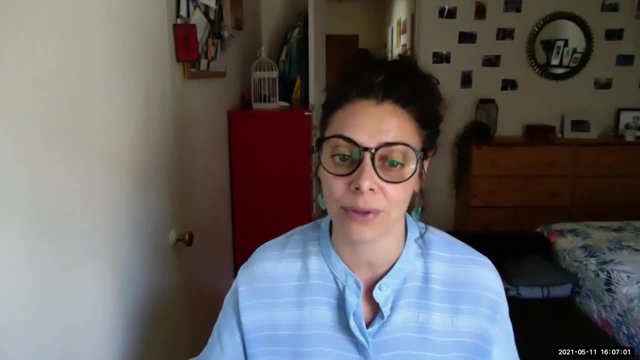 to introduce Dr Kira Borden. Kira is a- I would like to say, a good friend of mine and she is an answer postdoctoral fellow in the faculty of land and food systems, working with the sustainable agriculture landscapes lab led by Shana Smogler. She is an agro ecologist with 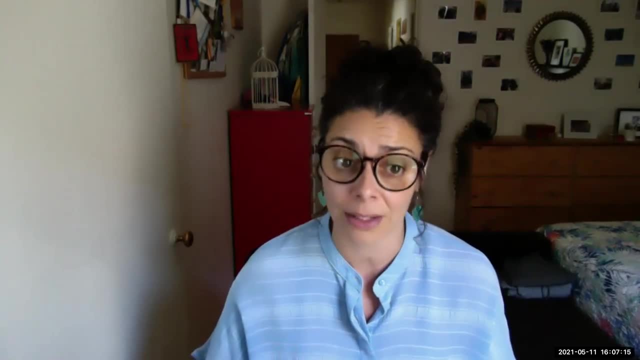 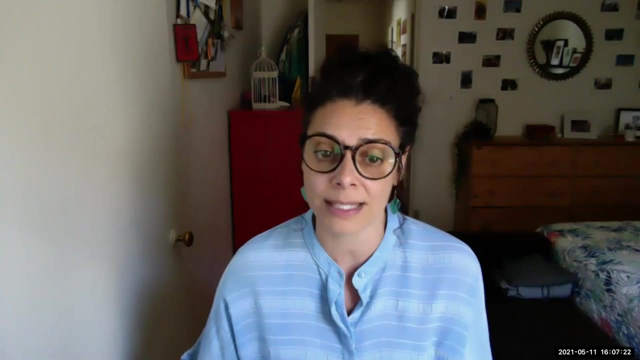 expertise in plant functional ecology, ecology and biochemistry, and Kira's research is centered on diversified agricultural systems of small and medium-scale farms, produced in a range of crops in temperate and tropical droughts. She is an expert in biochemical and chemical, organic and natural. 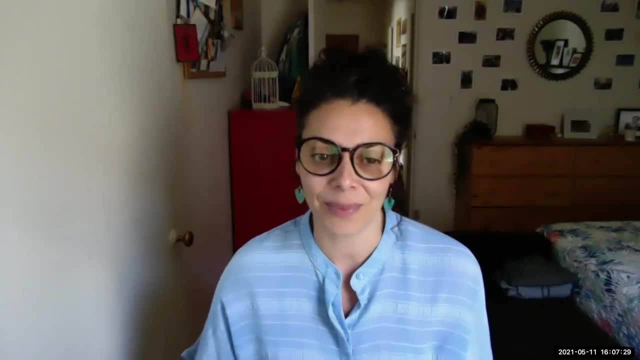 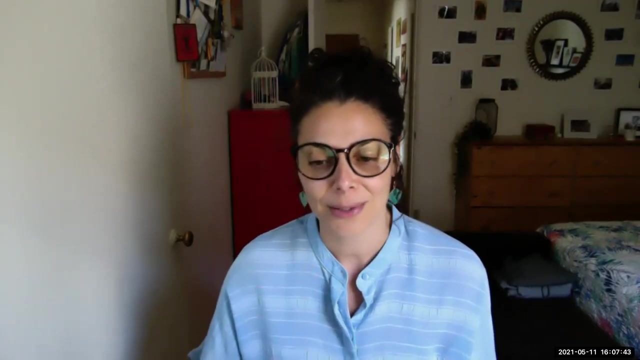 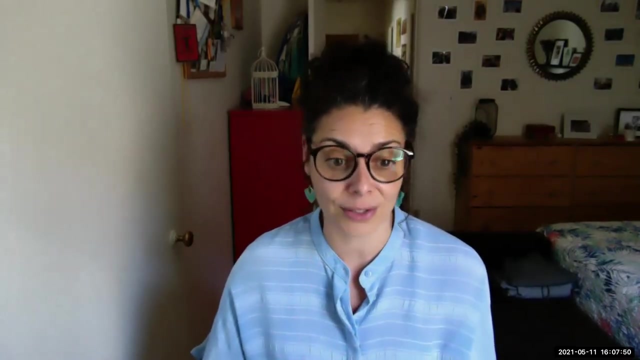 tropical regions later this year, um, and that's exciting news. and she will be investigating the below ground mechanisms regulating greenhouse gas emissions from diversified cover crops, um, as a banting fellow at the university of wealth. so congratulations, kira, for that new position. um, and yeah, and with that i think the floor is yours, kira. you can share your screen and start. 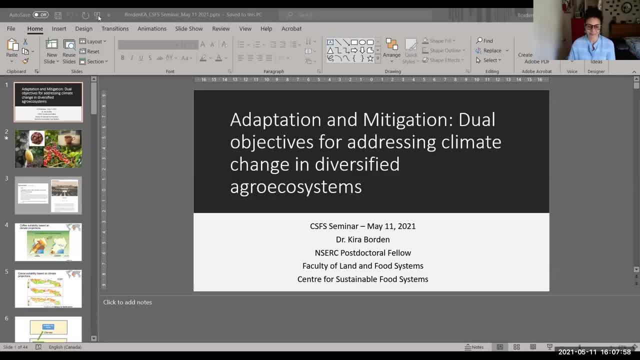 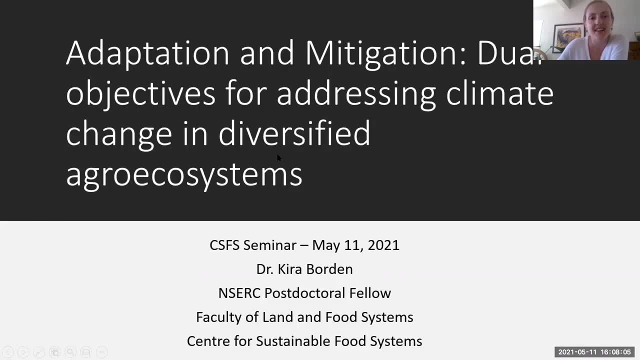 your presentation. thank you so much. thanks, lara. okay, it looks good. um, thanks everyone for uh coming to this seminar. i appreciate you taking your time, uh, during a beautiful tuesday afternoon, maybe some of you can listen in from outside, or at least with the window open. um, yeah, i think, lara, you gave me a great introduction. 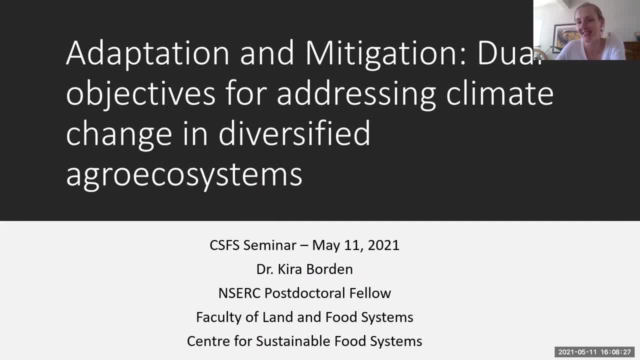 so i don't really need to give any background on myself and hopefully my research can speak for itself. um great, and thank you for the land acknowledgement, because i do do some research here in vancouver and on ubc farm. all right, so i'll start off with kind of a brief introduction. 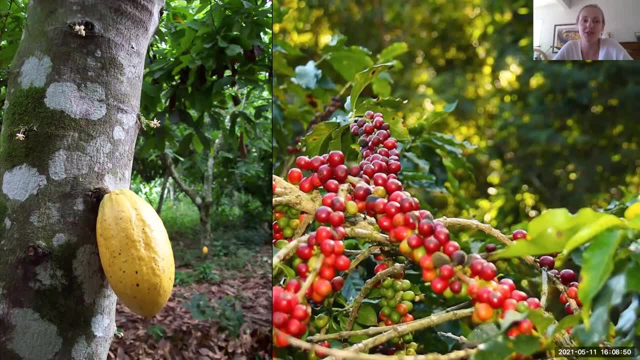 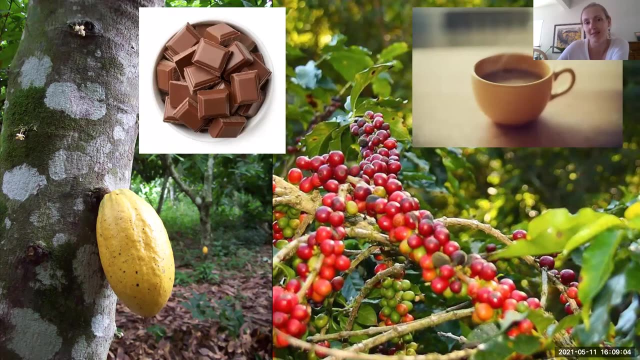 on on the topic of of agriculture and climate change. um, many of you probably recognize these tree crops that are shown. on the left is cocoa, so inside those pods are the, the seeds or the beans that produce chocolate, and on the right is a coffee plant with the cherries and. 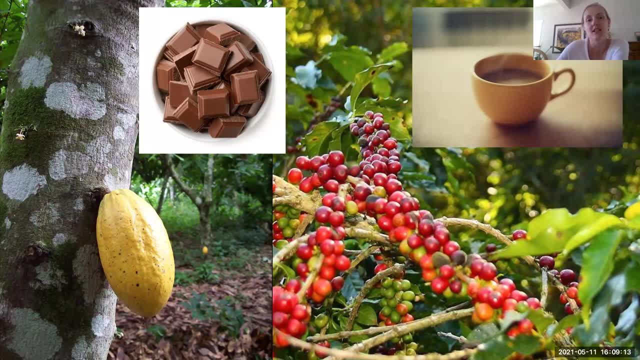 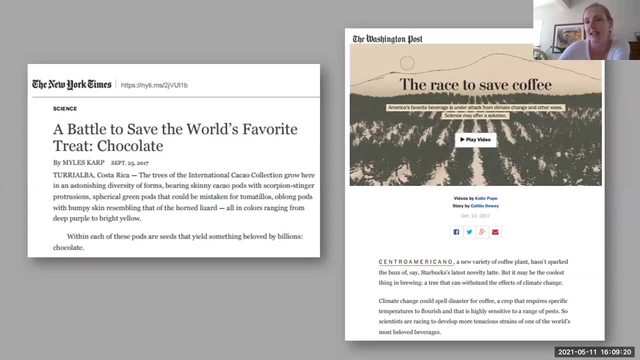 inside the beans that produce delicious coffee. so these two tree crops are tropical crops and they've been receiving a lot of press recently in regards to how they're going to get impacted by climate change, whether by direct impacts from changing climate, like precipitation and temperature or floods or drought, or indirect effects from shifting climate and pests, and 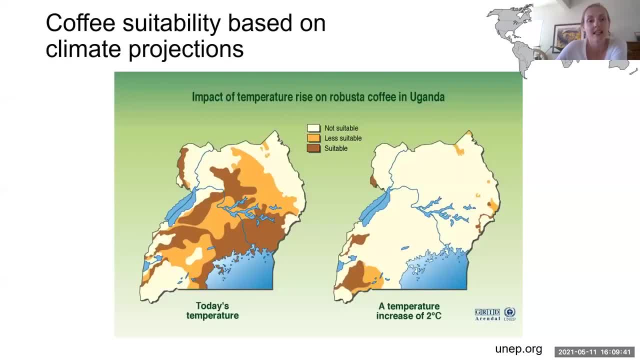 pathogen pressures and here's some uh projections of uh some you know, some negative consequences of climate change on on coffee in uganda from unep under a two degree increase scenario where we can see dramatic decline in an area that it's going to be suitable for. 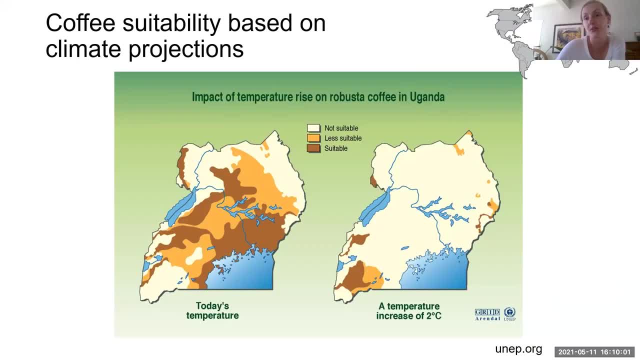 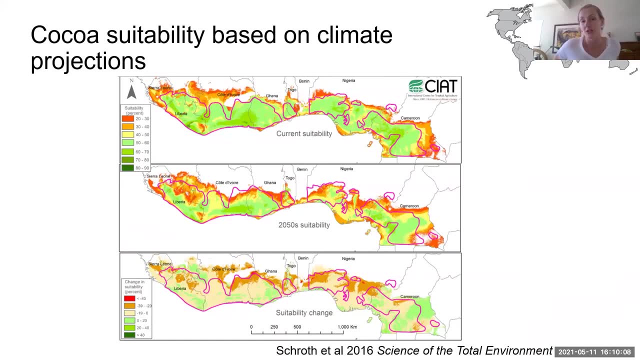 for coffee growing, based on their temperature and their precipitation requirements, and this is a little bit more of a detailed analysis done a few years ago on cocoa, which is a crop that i've done a lot of research on, and we can see at the top, you know, there's large, large. 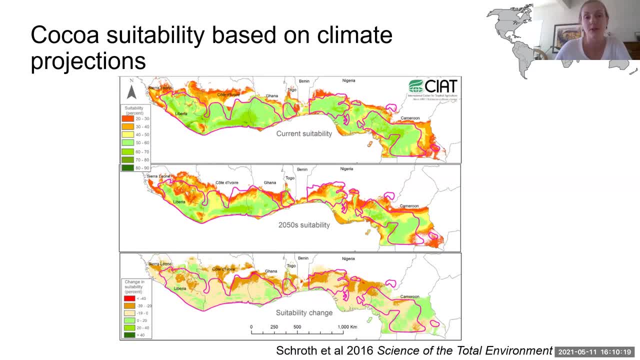 swaths of west africa that are climatically suitable for cocoa. um, and it actually is where the uh cocoa is produced in the world currently. uh, but under uh our- you know- climate change projections, uh, by the year 2050, uh, large areas will become unsuitable for the production of cocoa. 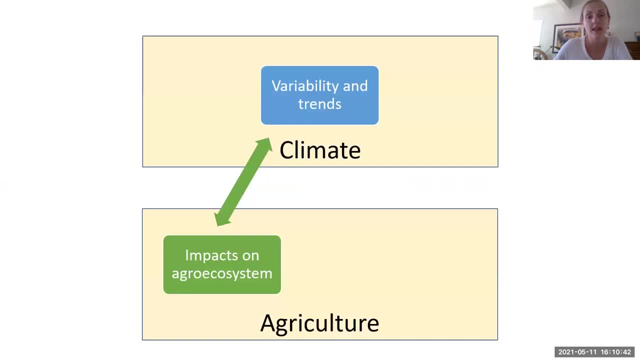 or for cocoa growth. so we have these direct impacts from climate on to agriculture and how plants can grow on different climates in the future, resulting from different variability and trends in precipitation and temperature. but of course, agriculture has a major role in contributing to anthropogenic climate change because of the emissions of greenhouse gases. 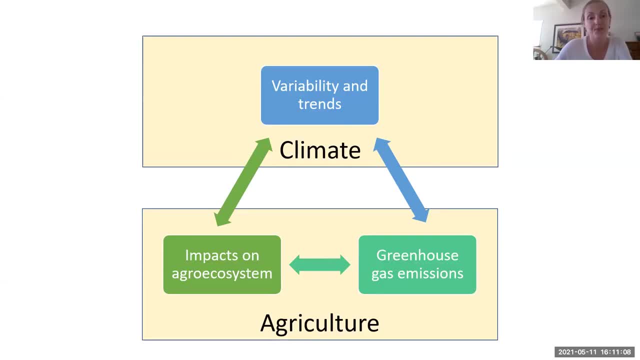 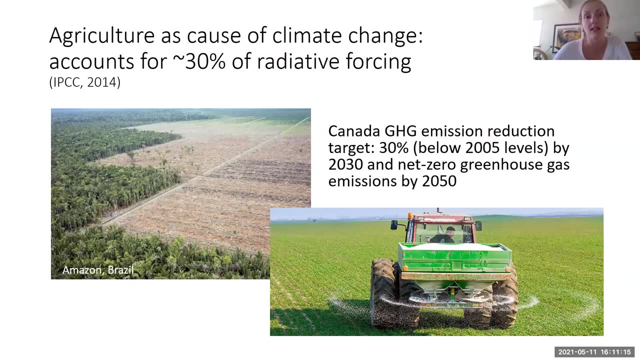 and losses of carbon to the atmosphere as co2. and on that note, uh, you know, agriculture is known to have cumulatively contributed 30 percent of radiative forcing um, and i guess, from a domestic standpoint, maybe a political point of view, but i think it's important to note that agriculture is 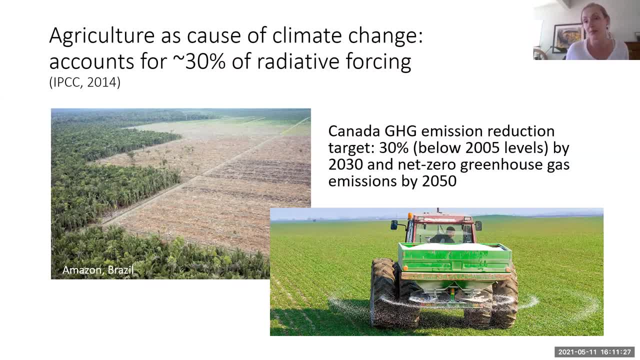 going to be a major part of the future. so just to give some general information, uh, we not only have a major portion of our commercial and industrial emissions, but we've been doing some babies and habitat management on agricultural systems. um, and some of our uh crops and species and soils and and, uh, you know, agriculture has been a major part of that. 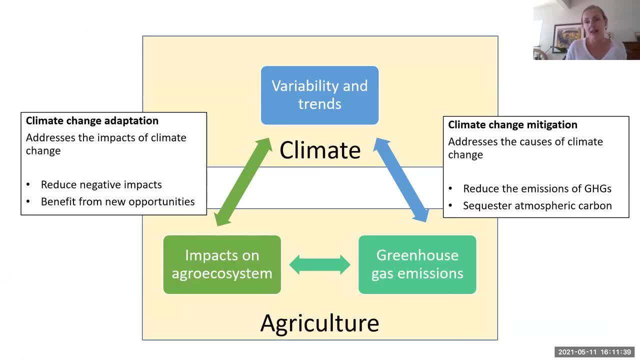 and we've very much contributed to the climate change across the fixtures. so, from a political standpoint, we've committed to reducing our ghg emissions by 30 for 2030, and that includes within the agriculture sector. so from these two angles of out of you know how. 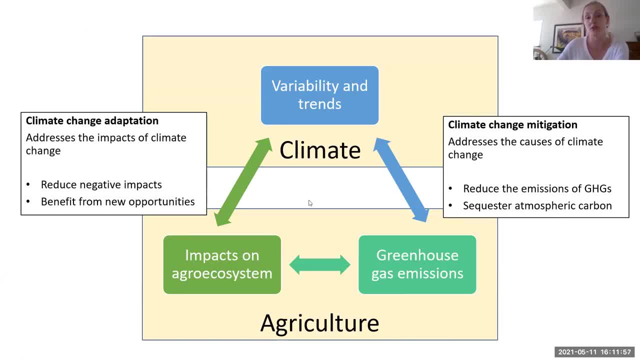 on our agro-ecosystems or from benefiting from new opportunities. And then on the other side it's: how can we reduce the emissions of GHGs or greenhouse gases, so methane, nitrous oxide and carbon dioxide, or reduce carbon dioxide in the atmosphere? 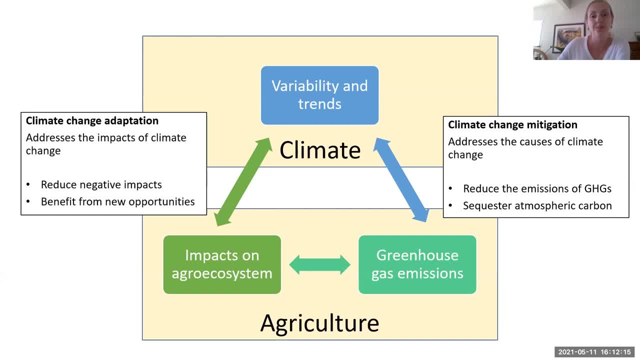 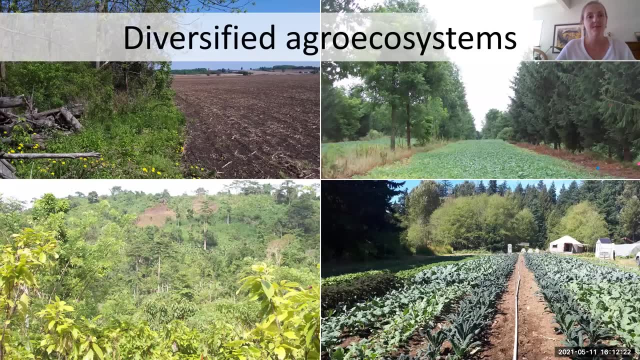 through sequestration of carbon. So how does diversified agro-ecosystems come into this? So these are some study sites that I've worked in from Ontario. along the top Bottom left is from Ghana And in the bottom right many of you, of course, will know that's UBC Farm. 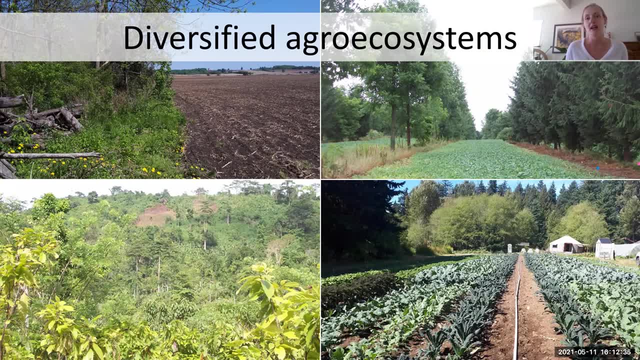 And so these systems have a diversity of crops, whether like where crops are being grown, or maybe integrated into the landscape, And the idea is that with higher diversity, we can achieve a higher ecosystem. We can achieve higher diversity, We can achieve a higher ecosystem. We can achieve a higher ecosystem. We can achieve. 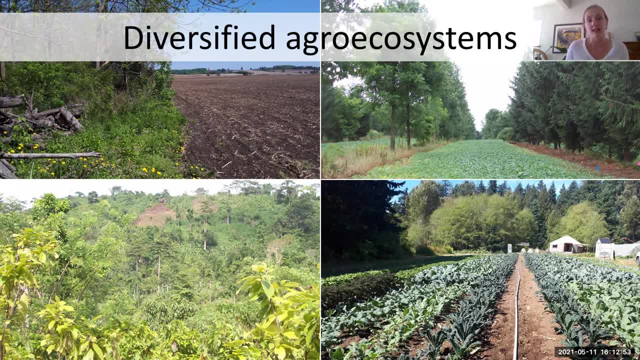 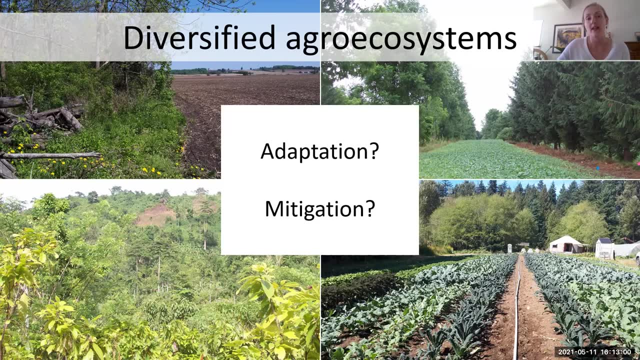 higher ecosystem services and function, And I'll get into that a little bit in a second. And then so, with that, as we achieve higher ecosystem functions, can that contribute to climate change adaptation and mitigation? So those are the types of questions, the big picture. 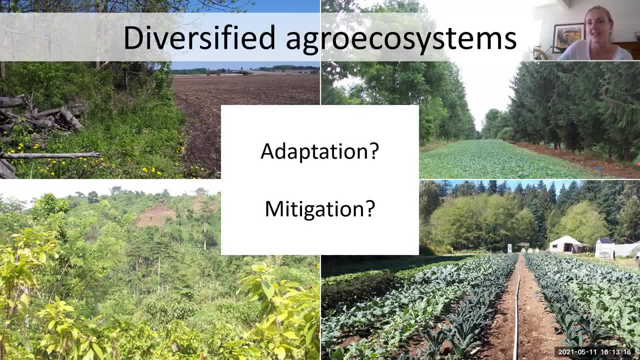 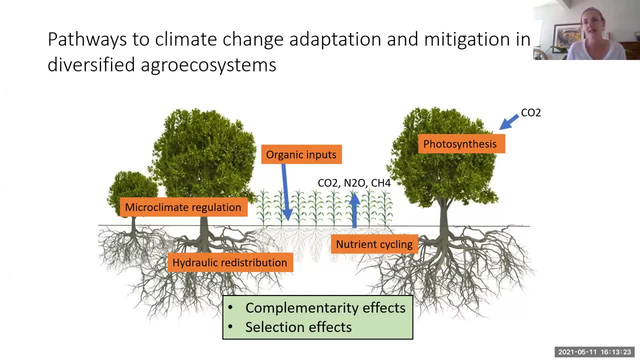 questions that inform the research that I'm going to give some overview of. So this schematic is showing a diversified system. We've got different crops, different types of plants with different functional attributes. They're growing in one location or perhaps maybe they're being rotated. 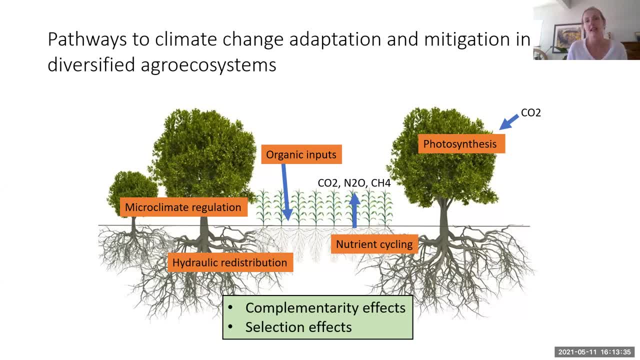 And the idea is that they have these different processes going on, And how could they be better than a monoculture system? Well, they could be. you know, there could be some kind of complementary or facilitative interactions that are occurring, So different crops are interacting and accessing different crops. 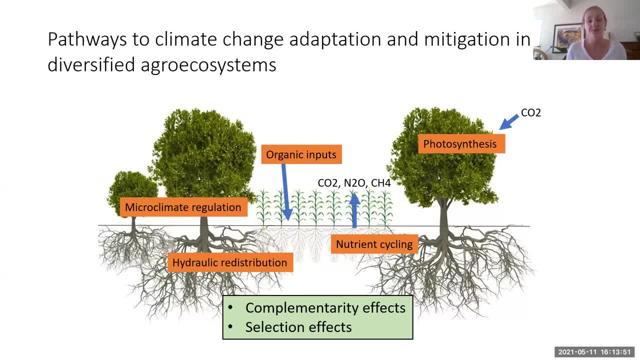 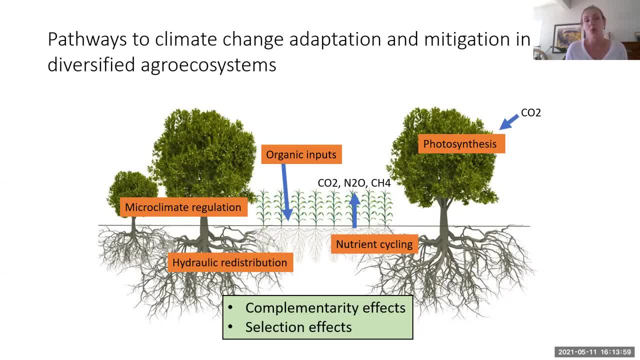 So we call that complementarity effects. Or we're integrating, we're selecting and integrating specific species that can, you know, amplify or can enhance some type of ecological function. So that's a selection effect. So those are kind of the two main pathways that we can achieve a higher 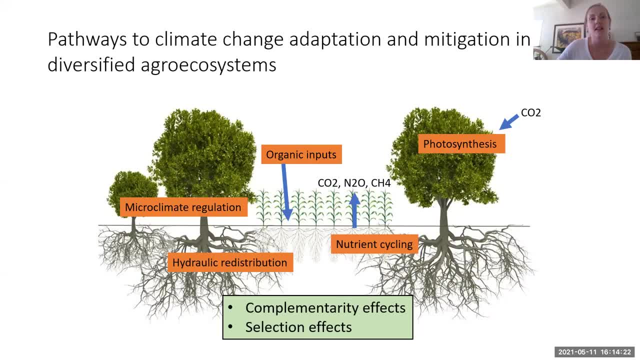 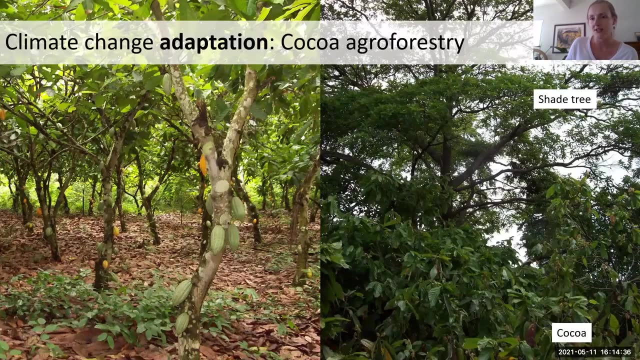 ecological performance on a system by diversifying the- you know, the farm or the farming landscape. So I'll start off with a couple examples of some research that I've done on the adaptation side. So my PhD at the University of Toronto, with Marnie Isaac as my advisor, I conducted my 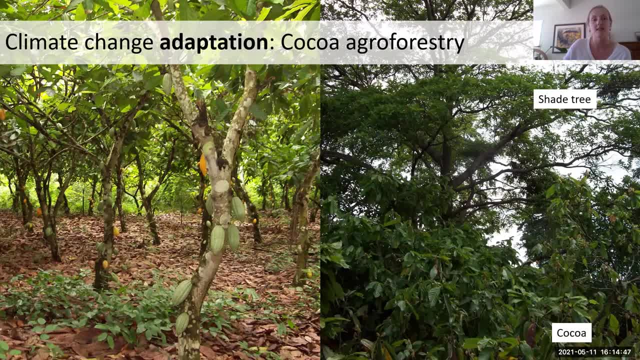 my research in Ghana on cocoa agroforestry systems, And so again, here's just some images of cocoa, the ambroma cacao, And we've got, you know, a bunch of cocoa trees on the left here, And then I took a photo kind of just above the cocoa canopy, And 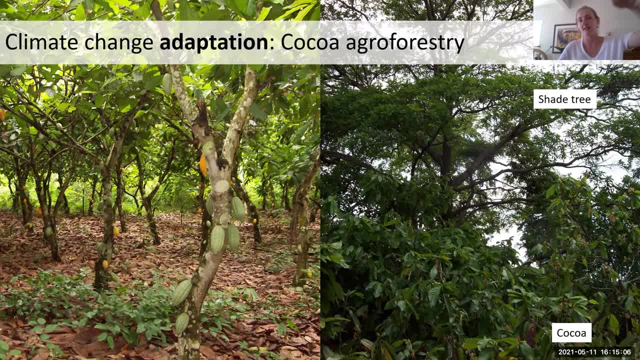 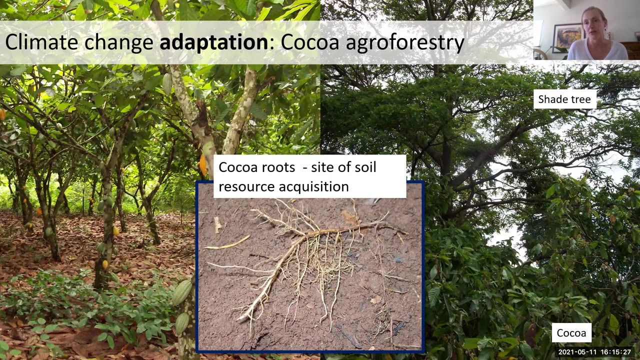 then you can see a shade tree. that's obviously shading the cocoa tree. So cocoa are shade adapted tropical crops and they can do well under shade systems. So they're already inclined towards these more like diversified systems, And my work specifically focused on what was going on below ground. So in this study that I'm going, 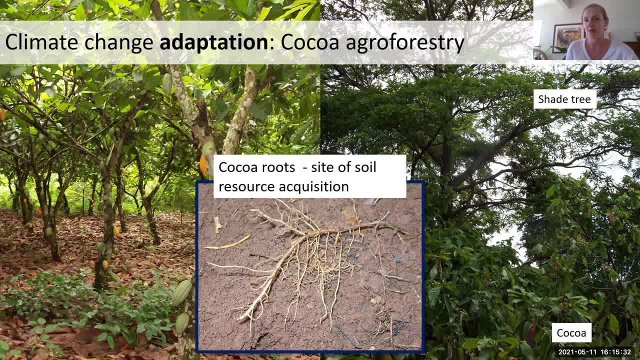 to describe to you. we looked at the root systems of cocoa to see how they're acquiring resources from soil. And so these crops- you know they're- they're grown by small scale farms or farmers and they don't usually use a lot of inputs. there's no irrigation generally. 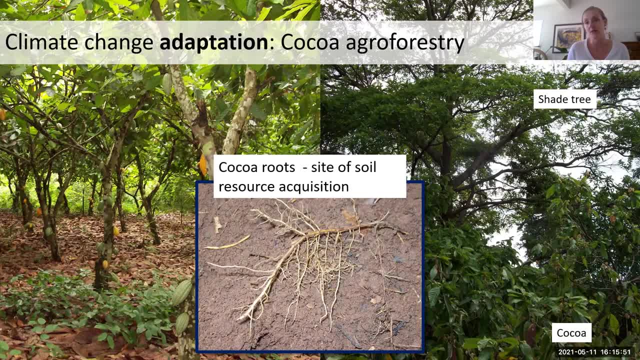 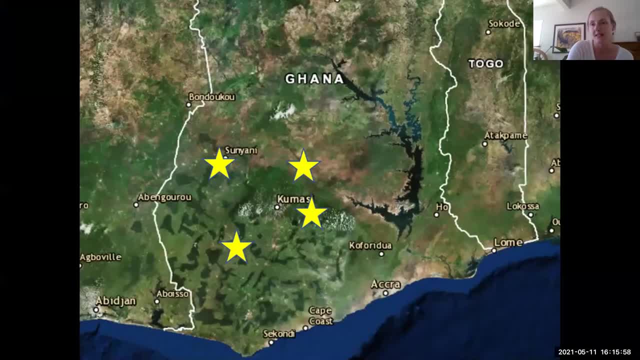 So really understanding how the crops are acquiring resources make some direct links to how well the crop is going to perform. And I went across these different sites So you can actually see. this is, you know, a bit blurry, But you can see where the green is. that's obviously where there's high rates of 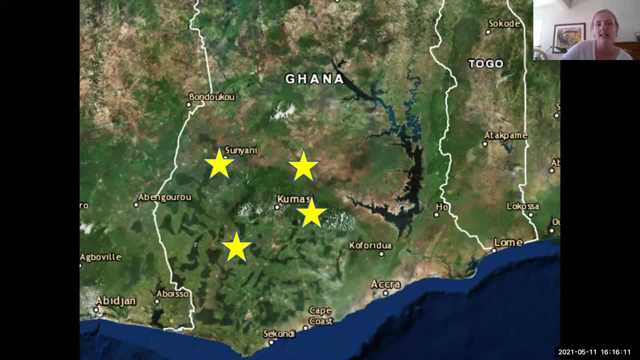 higher precipitation, more vegetation, more productivity, And it's in that area actually that cocoa is grown quite easily, And so you can see here that cocoa has grown by. I think it's kind of a half of an inch or so up to the middle of the vertical layer, And so it's, you know. you can actually see that. you can actually see that cocoa grows a lot of. you know maybe about 5,, 5, 6 hectares. That's about 1 hectare of of conical relative to the soil, And so you can see here that cocoa is growing quite, quite. 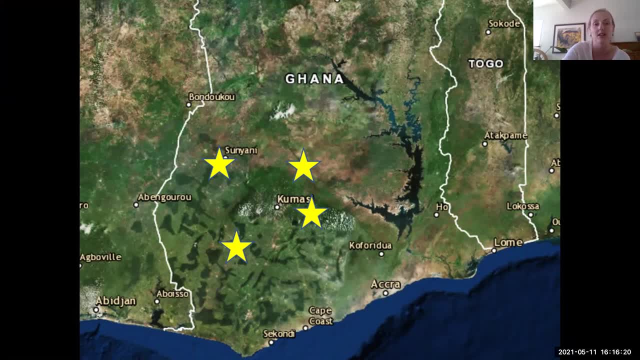 quite. i guess there's a lot of cocoa being grown in uh in ghana is what i'm trying to say. um and i picked areas that were in a well within that cocoa growing region, so they're meeting the climatic requirements of cocoa, as well as a couple that um are up here towards what we. 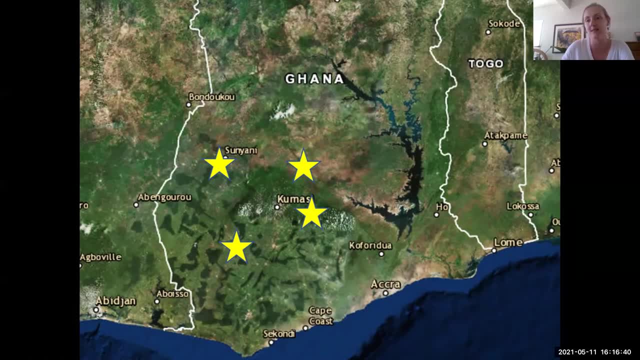 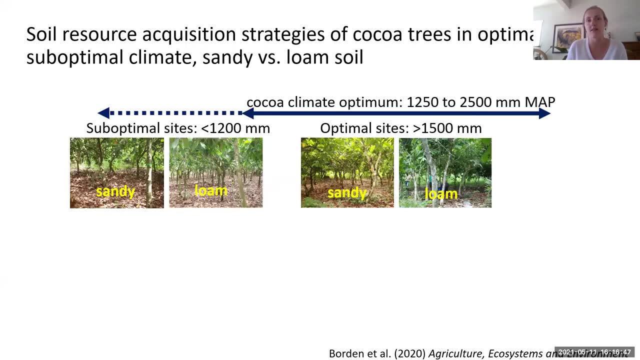 call the transition zone. so it's getting closer to the savannah and it's much drier. so this kind of summarizes that, that sampling scheme that i just described, uh. so it's looking at cocoa trees, uh, that are in that climatically optimal range, uh, and then 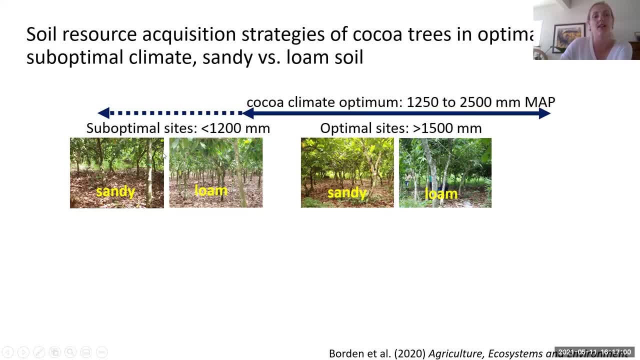 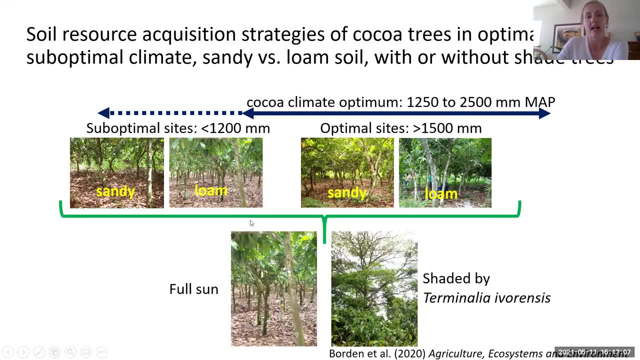 those that are getting closer to the transition zone in the north, that are in the sub-optimal uh precipitation range, uh oh, and then within that uh scene, there's was two different soil types. Sorry, I have a five-month-old right now, so I have a bit of a. 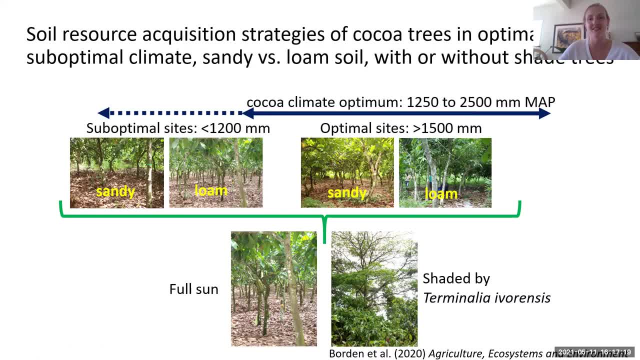 baby brain, so you might catch me a few times realizing that I've just forgotten to say something. So there's: within the two climatic zones we have different types of soil, so the idea is trying to get a little bit more nuanced information about how cocoa are responding to climate, based on some 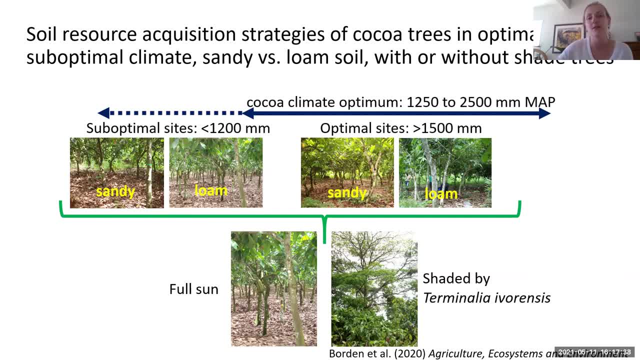 of the underlying growing conditions that they're on the soil properties. So we've got sandy and conditions and then, within each of those sites, areas where cocoa are grown, monoculture, versus those that are grown with Terminale ivarensis, which is this really big and commonly used timber. 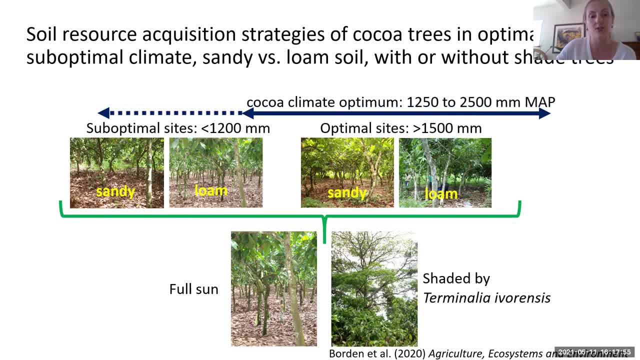 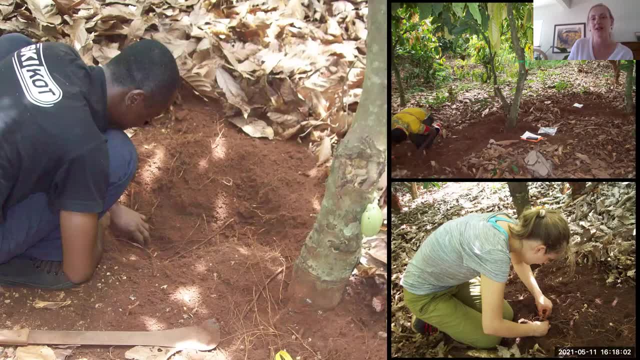 species that are used for shade in cocoa agroforestry in Ghana, And here myself, obviously in the bottom right, and then two colleagues, research assistants, that I hired from Kwame Nakura University of Science and Technology from Kumasi in Ghana. They were great and they helped me do these very labor-intensive. 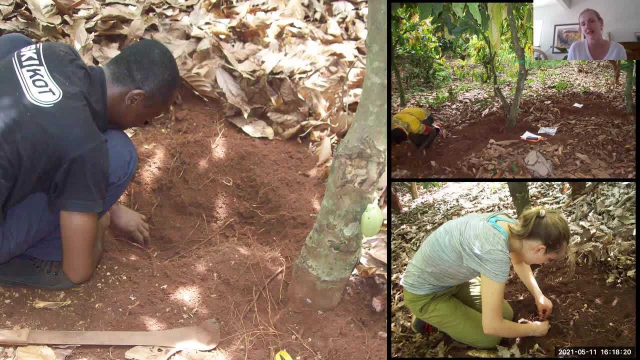 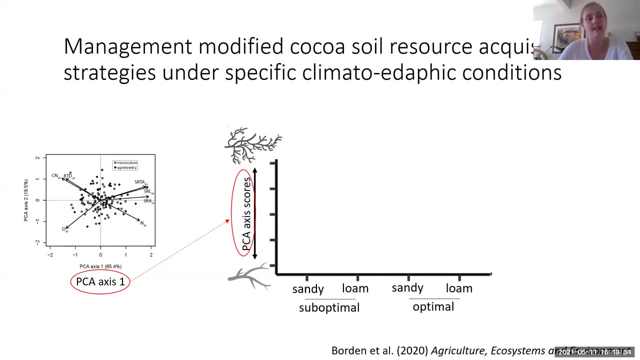 excavations of the roots. The idea was we had to, you know, locate roots that were directly attached to specific cocoa trees. So this is pretty, as you can see, back-aching work And from that, those samples. we conducted some analyses on their morphology and chemical. 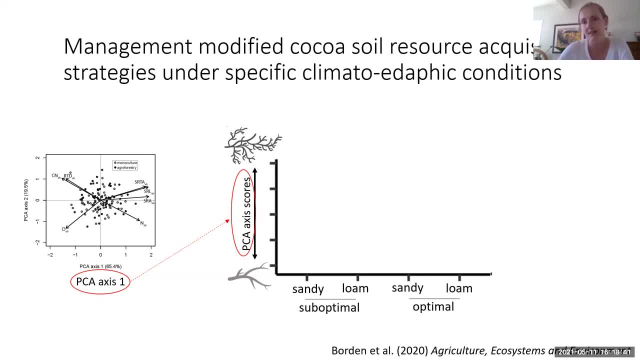 attributes that can tell us, you know, what's going on in the soil, what's going on in the soil, and then thank you to so and so- and ourselves also harder- uploaded these archaeological Political Reports. We have been doing near and heart research on this. as far as telling us something about how they 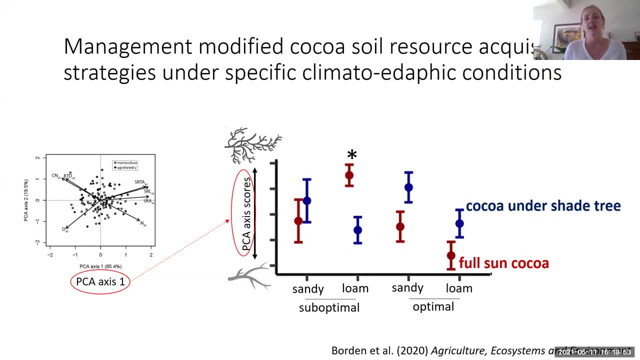 require resources from from the soil And using those data, we looked at: Okay, so are they performing across different sites and with different management treatments, And so our analysis revealed that it's very context specific of of how agroforestry practices can modify how cocoa are going to be acquiring resources from soil. 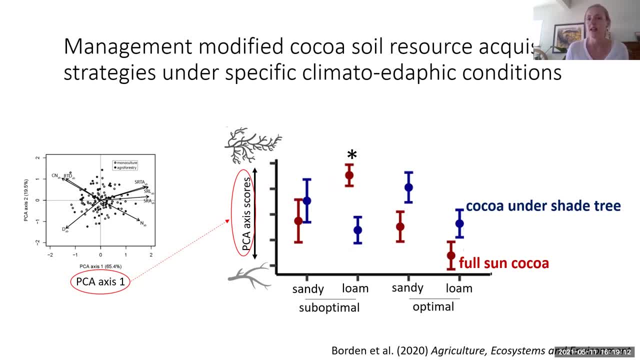 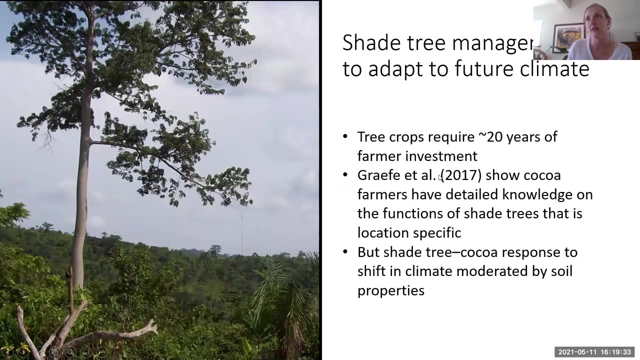 Me. we really saw a strong response of cocoa to being grown in agroforestry or being grown in monoculture, And so this can have implications of, you know, choosing shade tree species for adaptation purposes. And then I guess also it's conceptually or it's very practical to think about. 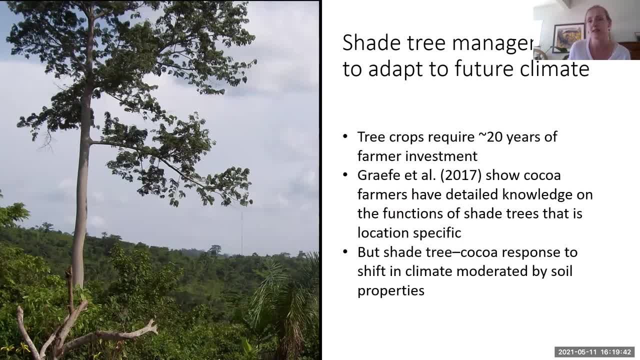 tree crops because you know farmers are going to invest in them for 20 years and so you know the climate that they grow them in now. it's going to be vastly different, or could be vastly different, in 20 years from now. So the the whole time scale of climate change is very real. 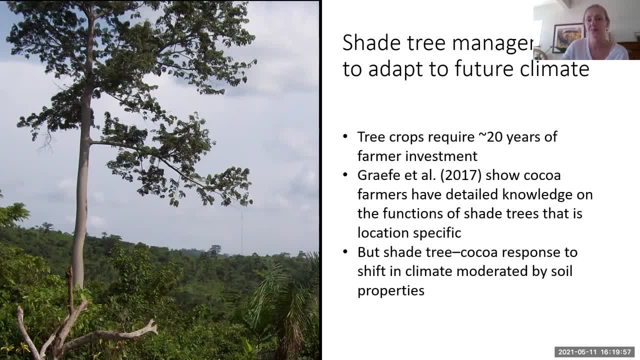 for for cocoa farmers and other farmers who work with tree crops, And other researchers have done fantastic work looking at how much knowledge or the knowledge that farmers have- and they already are selecting shade trees that are, that are conducive or that are good for their research, And so I think it's really important to think about that. I think it's really important. 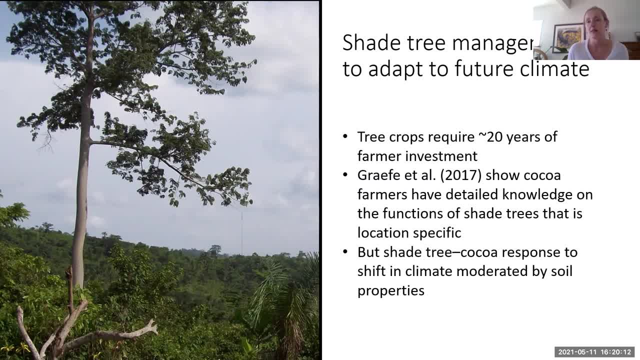 to think about that. I think it's really important to think about that. I think it's really important- perspective climates, but of course, as that changes, they need you know new practices to adopt And so, knowing that there's these context, specific requirements like maybe you need to consider, 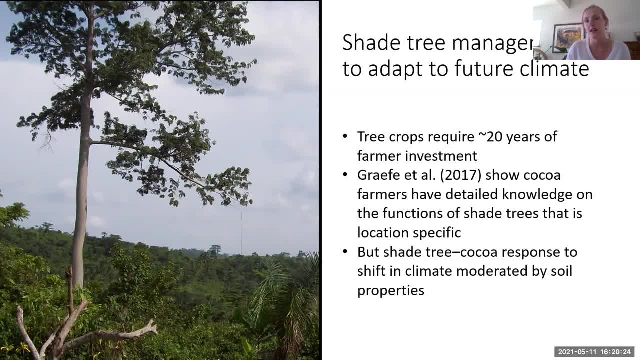 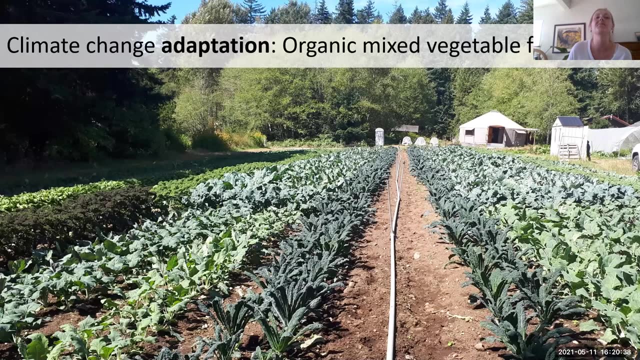 the, the soil texture, when you decide on if a specific shade tree is going to be good in the future. Those are the type of information that this type of research would help to inform. so then, if we're shifting continents, um, Um, this is the work that I've been working on at UBC farm, So we're looking at mixed vegetable farms or organic vegetable farms in BC. these are small, medium scale farms. 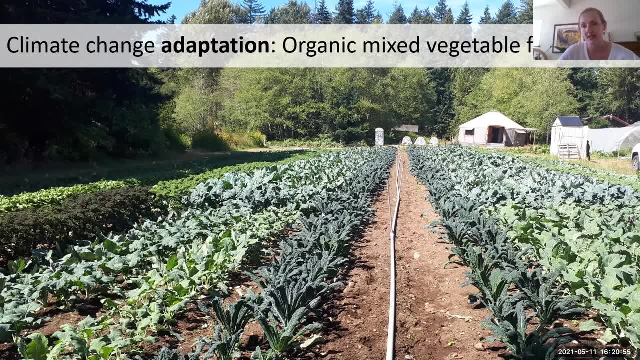 And that you know are growing a diversity of crops over different years or, as you can see, at the same time we've got different brassica species growing together- cabbage and kale and cauliflower- And so for this research that's been initiated. 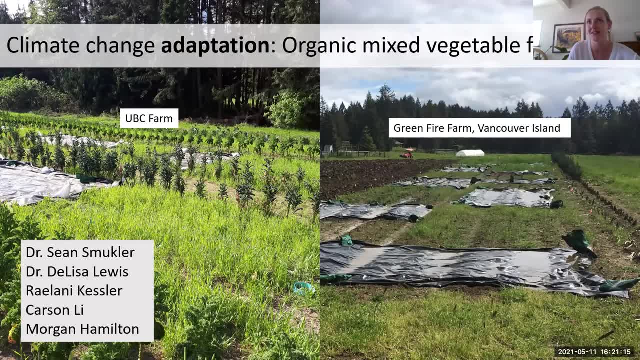 I guess a year ago, two years ago, We set up this experiment to to see how, over winter, precipitation can be better managed on these farms. so it's expected that there's gonna be more precipitation in in the area On the shoulder season, so in the spring and the fall, And so this makes managing these these farms a little bit more difficult. 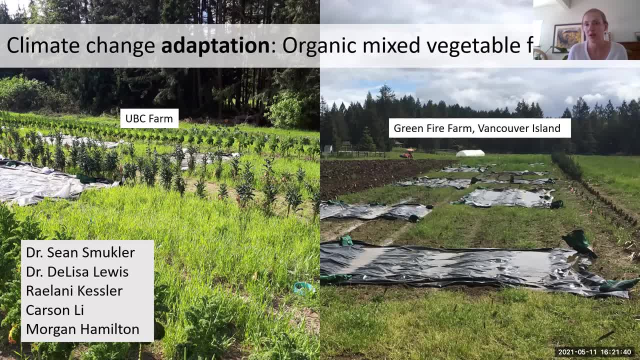 And so this makes managing these these farms a little bit more difficult, And so this makes managing these these farms a little bit more challenging. and so looking at cover cropping systems or plastic mulch as a way to regulate some oysters is the broad objective of this research. 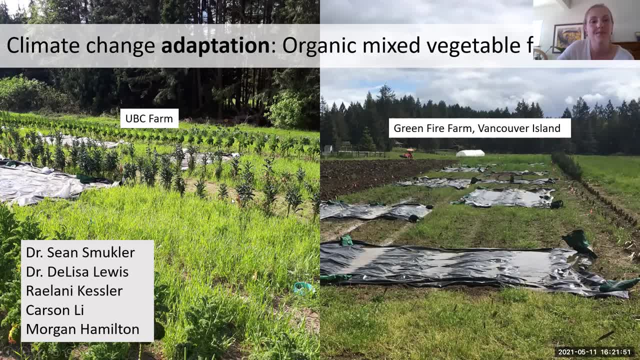 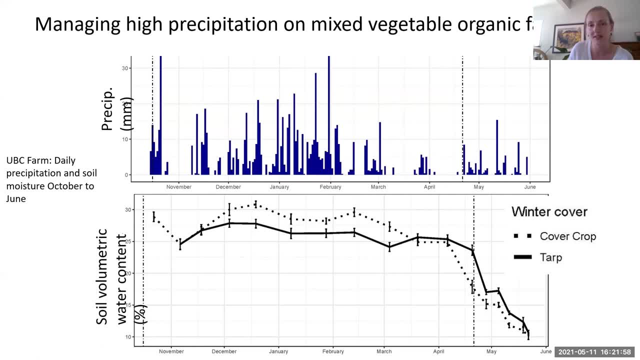 And I've listed the main researchers that are involved in this project And so that you can see on the top as precipitation over the year, where these big bars of blue of our high precipitation events occurring predominantly in the winter months. And so these are just some examples of our treatments on the soil. moisture conditions. 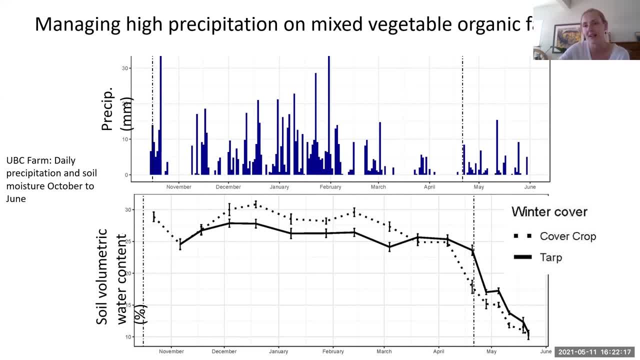 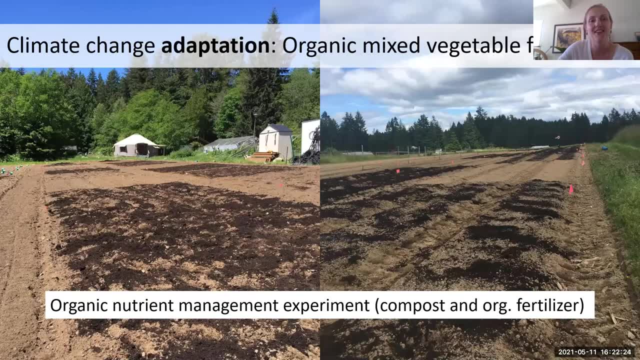 Under your cover, cropping or plastic mulch. So these are very preliminary results, just kind of characterizing how our treatments are impacting the soil environment for for these crops- And I've got a mountain of data that are waiting for me when I returned from that leaf- 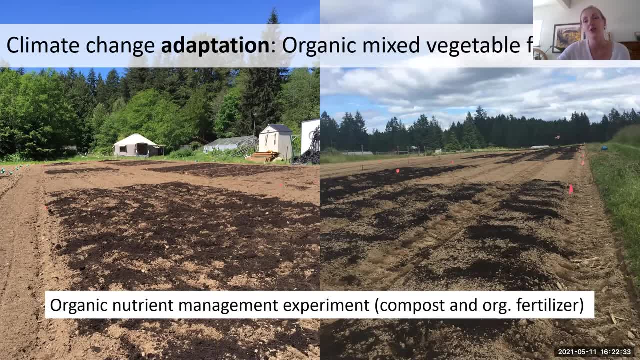 But I guess one of the interesting angles of this is that there's also, at the same time, this nutrient management practices as well. So organic farmers, you know, have lots of decisions to make, including how are they going to meet the nutrient requirements of crops and that ensures that they're organically. 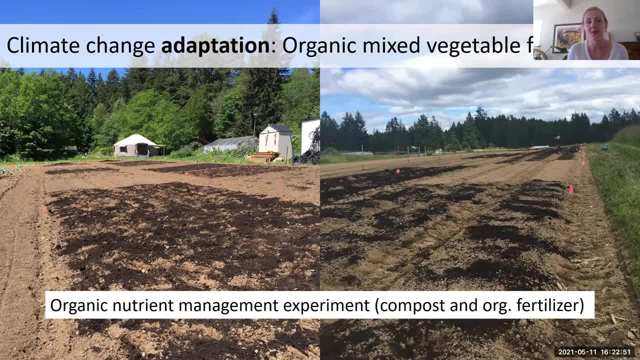 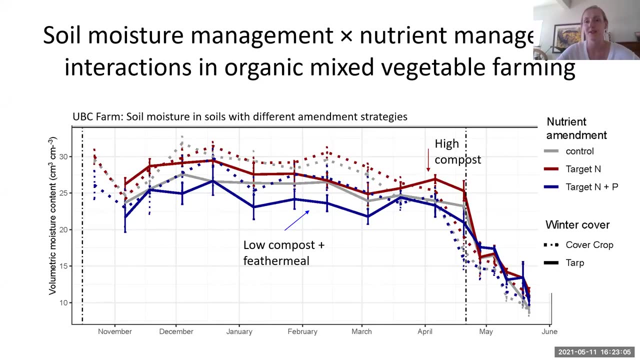 certified and building good organic matter in the soil, etc. So these pictures show some nutrient management trials or treatments being applied to the same sites And we're seeing some interesting interactions between our soil management treatments and the nutrient management treatments that are in place, And so I'm looking forward to kind of digging into that And it kind of ties. 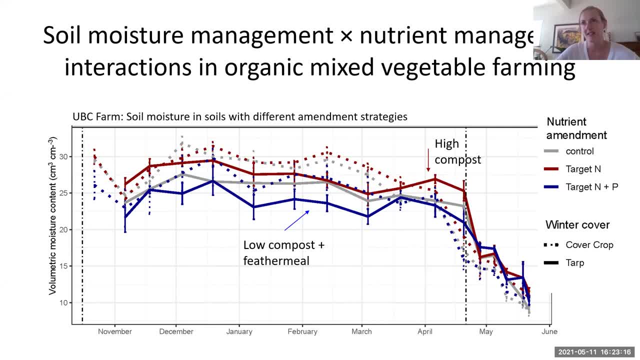 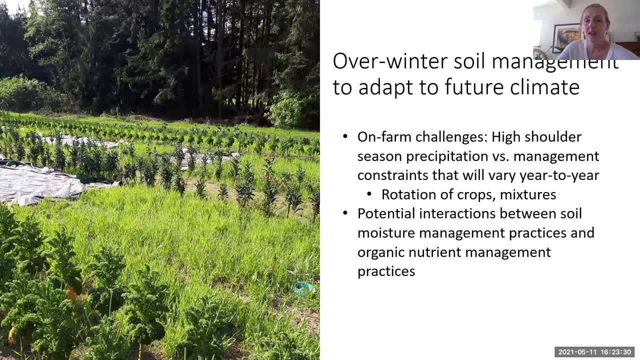 back to the other study, in that you know there are these kind of interactions between the soil conditions and these management practices in terms of soil moisture and, potentially, nutrients and how crops are going to be acquiring those nutrients. So the on-farm challenge. 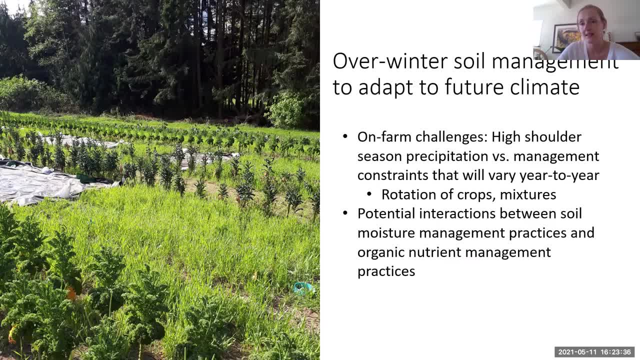 just again highlighting that, yeah, these small-scale, medium-scale farms are challenged with these high precipitation shoulder seasons, or increasingly so into the future, And that they're also. you know they have lots of constraints around. you know they have to make. 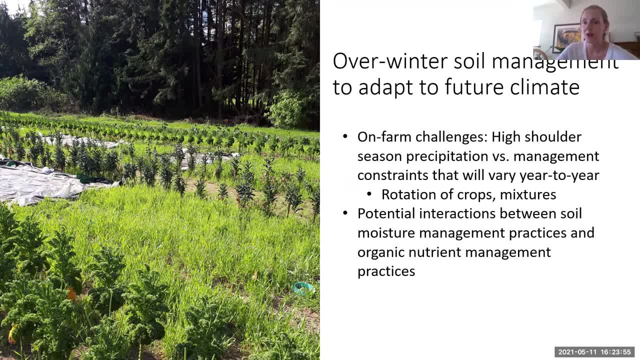 decisions? Can they establish cover crops? What crops are they going to grow the subsequent year? They're rotating crops, There's a mixture of crops which makes it very difficult to prescribe, you know, a single type of management. And then there's these potentials for interactions between 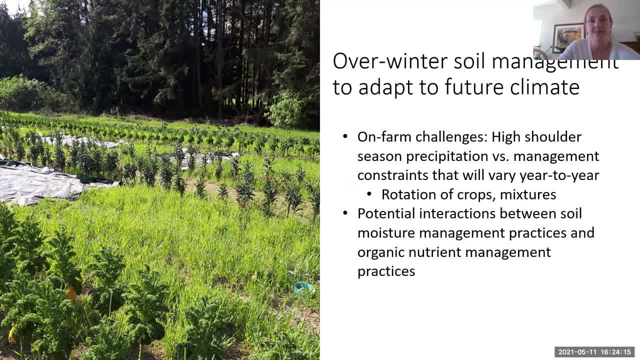 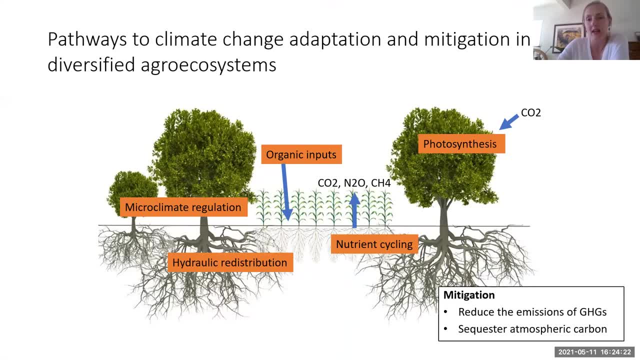 soil moisture management and nutrient management practices. So now shifting to the mitigation side, And so for this there's kind of two angles here. the one is to sequester atmospheric carbon, and so the first study that I'm going to describe really focuses on that. 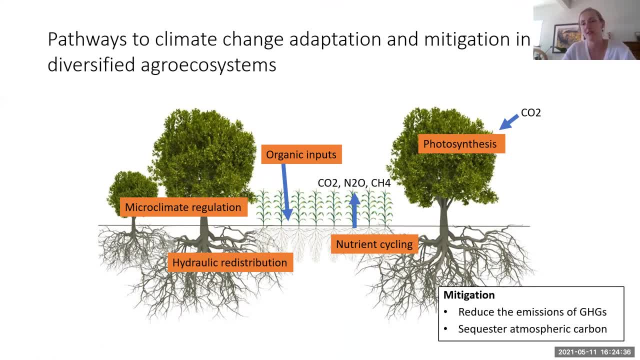 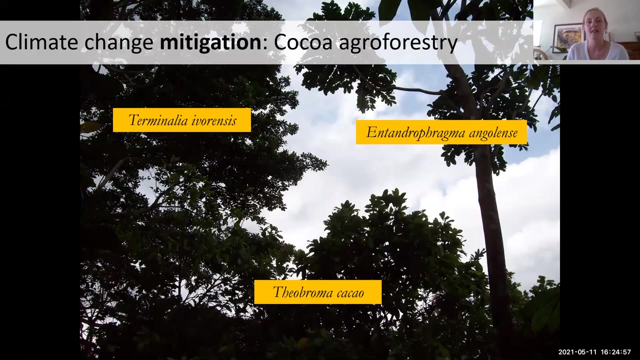 and how carbon is, you know, stored into crop biomass or tree biomass on a farm? and then the next one, or the subsequent studies, I'll talk about the emissions of greenhouse gases from soil. So back to Ghana and our cocoa agroforestry systems. obviously you know, if you, if you're. 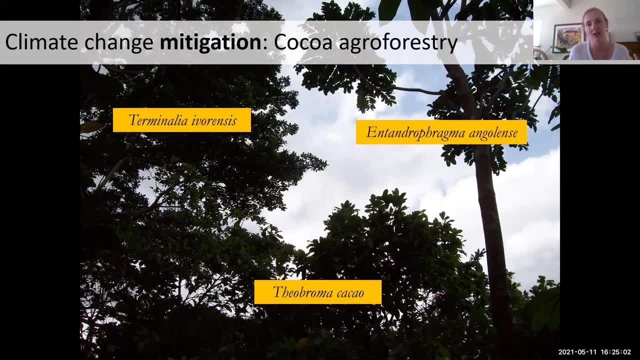 growing trees and these larger shade trees in a cocoa system, you're going to expect that you're going to have more biomass, carbon that's stored in those, those trees, right, so you would. you would see that as a carbon sink more so than a monoculture system where it's just cocoa. 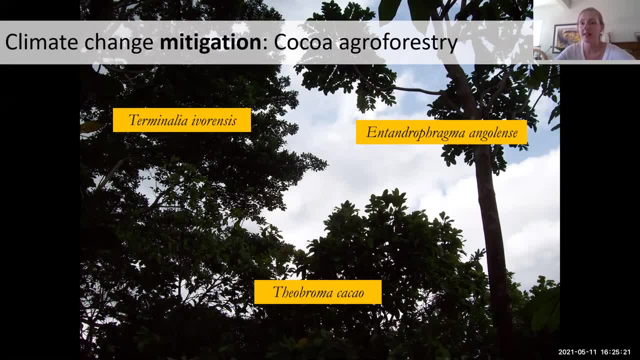 But of course we we lack data on what that. you know what those gains are and the nuances of what happens when you plant different types of species together, or you know what those gains are. So, yeah, what type of mixtures can be optimal for that type of mitigation objective? 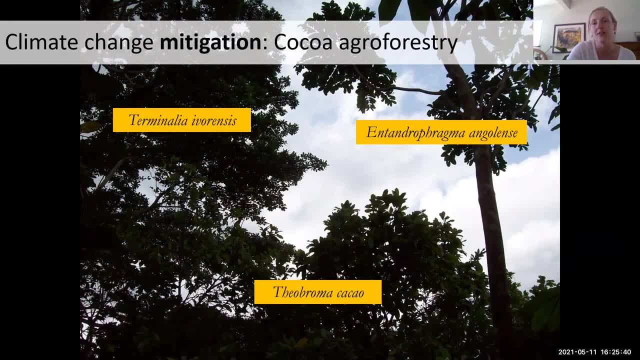 For this picture. you've got the Ambroma cacao and two different shade trees that are common to West Africa: The Terminalia, which we already talked about, that really big shade tree- it's a semi-deciduous- and then the Antodifragma angolensi, much different type of 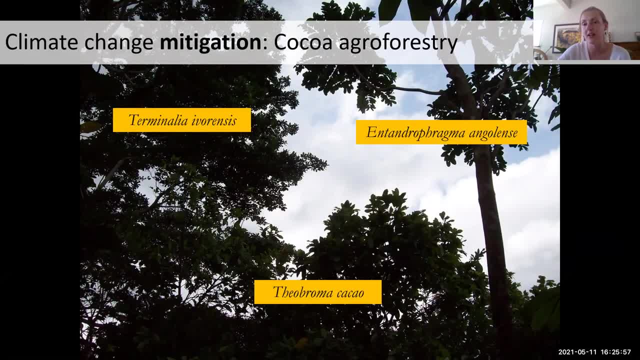 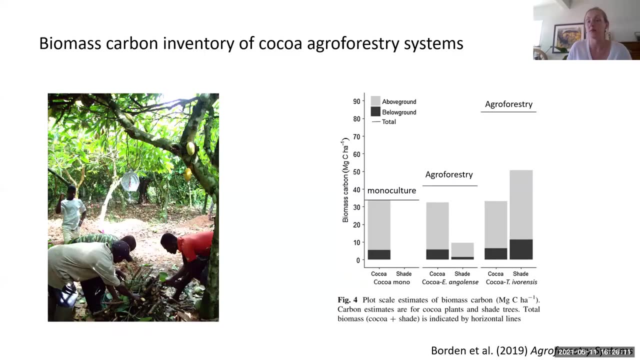 canopy structure a little bit more sparser. It's slower growing. you know a hardwood species, so they have these different functional attributes as well, the different shade trees. So here's some results from a study where we, you know, estimated how much carbon is in the biomass. 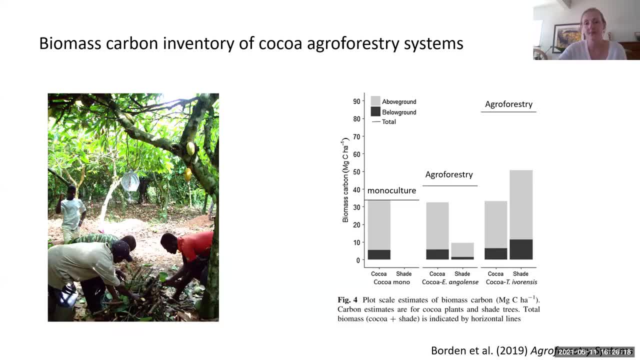 of these different systems. So monoculture- I overlaid it with the totals here- Monoculture obviously has lower. but then we have these two forms of agroforestry, so cocoa integrated with that slower growing hardwood and Antodifragma angolensi, versus cocoa integrated with those. 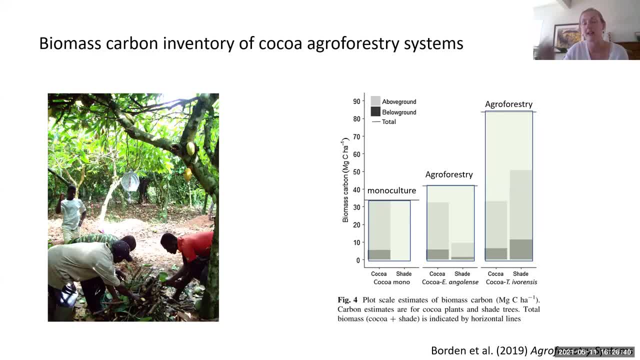 very fast growing pioneer species, the Terminalia ivarensis. So really no surprises in the. you know the results, but it's great to have these, these types of carbon data for these inventories. I guess one of the interesting sort of ecological outcomes of this research. 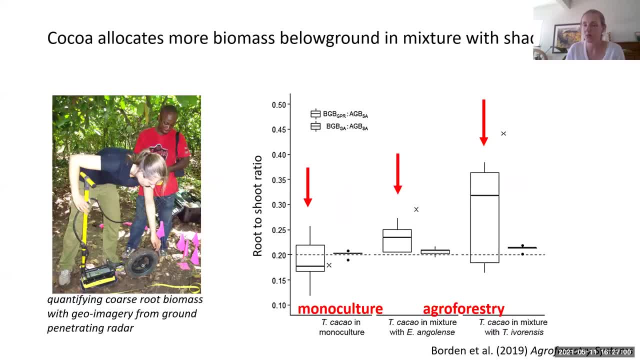 however, it shows that, based on whichever agroforestry practice the cocoa were growing in, they actually allocated biomass differently. So normally what we do is we go into to tabulate how much biomass and carbon you'd go in and you'd use these allometric equations. 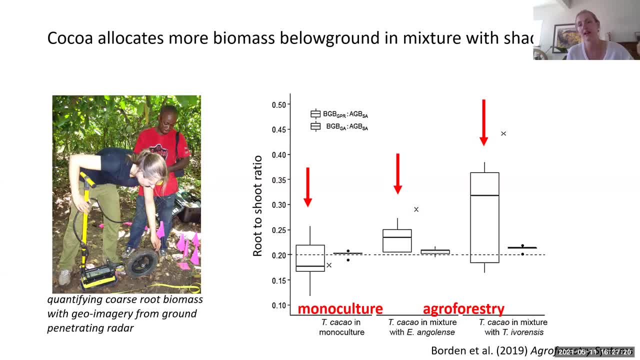 So you can measure the diameter of breast height, you can look at the tree height and we have these equations that tell us that can estimate the volume of wood that's there and we can apply a conversion to carbon. But what we found was that these allometric equations were not that. 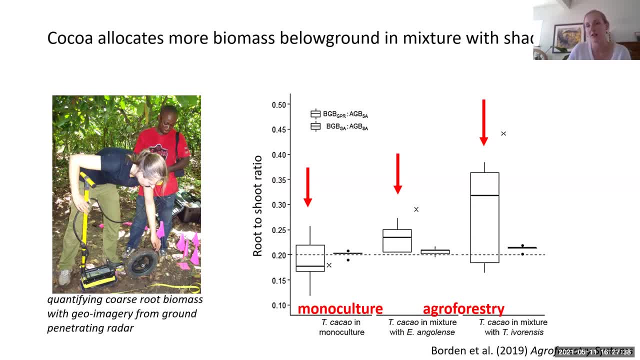 reliable for cocoa, based on whether they're being planted in monoculture or planted in an agroforestry system. So they're growing differently. they're growing more roots in the agroforestry system. so this is kind of a if the these boxes here. 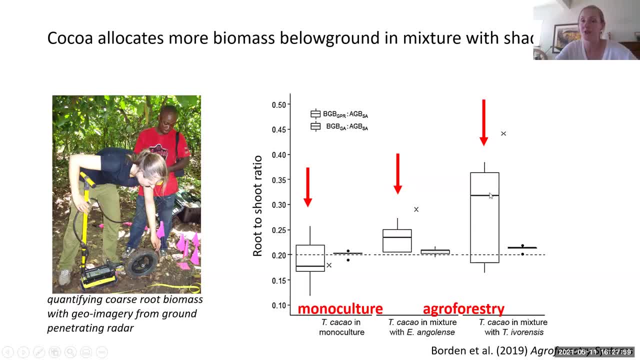 The higher the median is, actually higher the root tissue ratio, so more roots versus above ground biomass and it there's a lot of variability as well as, if you compare it to what you know, the IPCC or average amounts that would be calculated by allometric equations. 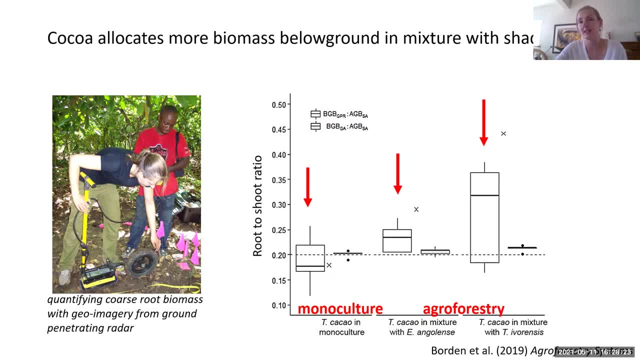 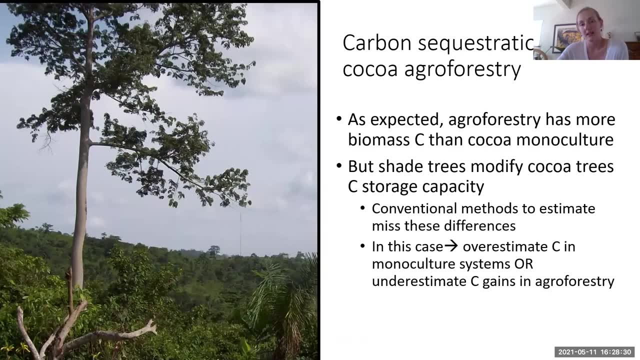 There's some, you know, misdifferences that conventional method methods lead to. So, like I said, as you expected, there's more carbon in agroforestry systems, but there is some nuance there and conventional methods might miss these differences. So on a farm scale these differences might be small. maybe you know a ton of carbon difference. 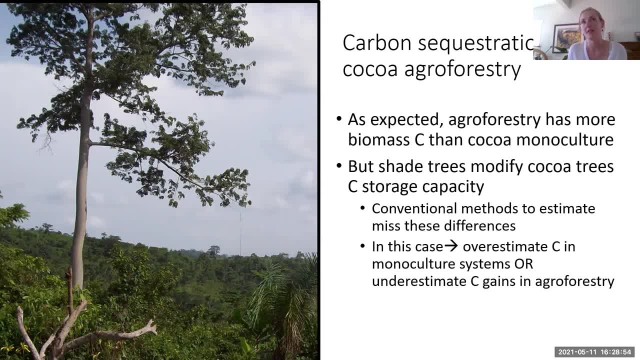 but then you start to extrapolate that to that, there being 1.6 million hectares of cocoa cultivation in Ghana, and you start to see that you know, if there's any kind of systematic variation occurring, that it can lead to these large differences in how we're accounting. 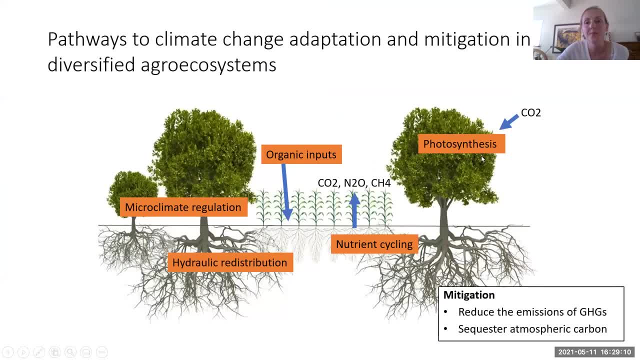 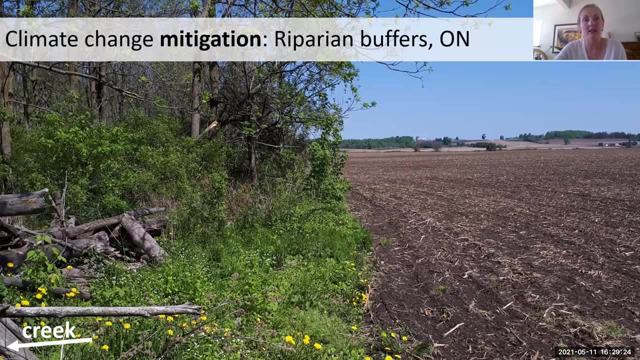 for carbon. Okay, so then that was the the carbon sequestration side, flipping to the emission side of mitigation. This work that I'm going to start with it's back in Ontario and we were looking at, so this is part of the agriculture greenhouse grasses program. 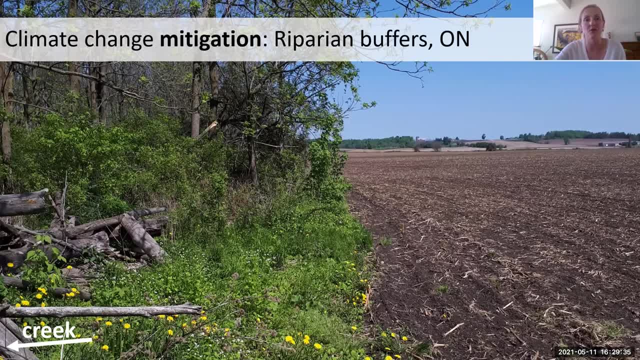 project that I was involved in with the University of Guelph and University of Toronto, and we focused on riparian buffers in the Guelph area, and so these, these buffer systems, as many of us already know, are ways to mitigate impacts from from agriculture. so in the case here, it's intensive corn and soybean rotation in Ontario. 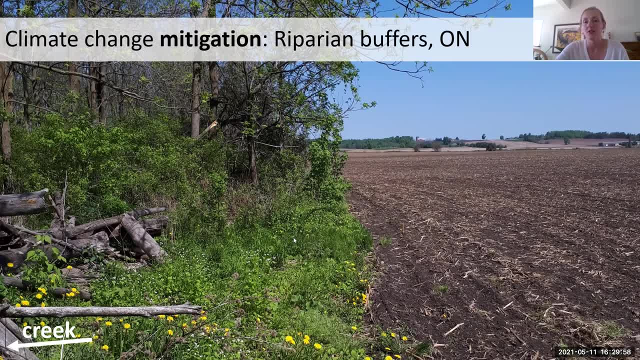 So mitigate the impacts of, you know, nutrients leaching into to waterways and just stream banks. it's a source of additional biodiversity, microclimate regulation of the stream. there's many ecological benefits to these, but there's not much known about what type of impact they might have on the mitigation. 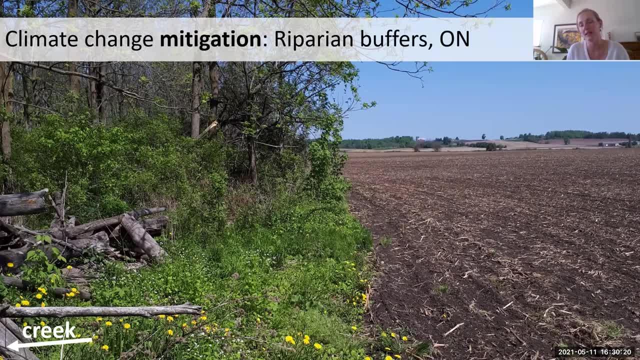 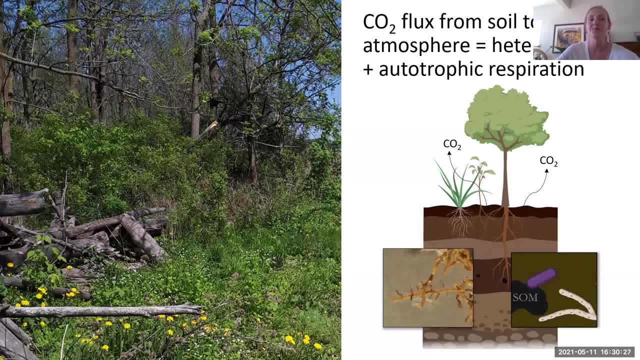 capacity of our landscapes, and we really, for this work, dived into the nitty-gritty of what's driving CO2 emissions from soil. so soil respiration is a function of basically two components: what's coming from autotrophic respiration below ground, so root respiration- and what's coming from 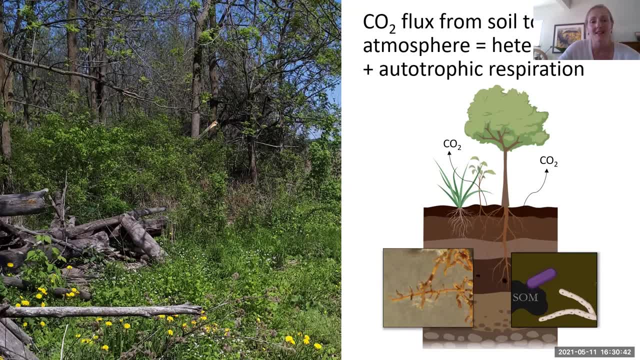 heterotrophic respiration, and so we we wanted to understand. you know we looked at different types of riparian systems and wanted to understand, well, what's contributing to overall cell respiration rate. is there a way to understand the, the drive, you know the, the main factors and what's driving CO2 respiration and this carbon flux to the atmosphere? 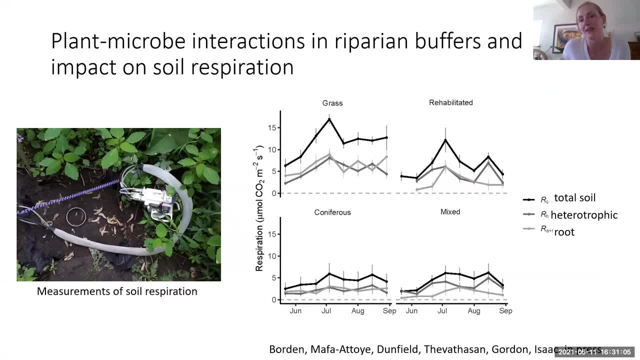 So I'm not a soil microbiologist, so we worked with soil microbiologists to answer these types of questions. We set up these root exclusion experiments in order to try- and there's limits, but it's a way to try and tease apart carbon dioxide that's coming from roots versus 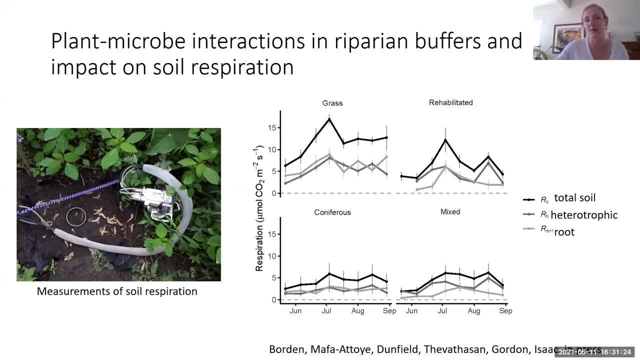 what's coming from autotrophic respiration from the microbes and soil, And so these data are the four different types of riparian buffers that we worked in: a grassland buffer, a rehabilitated tree buffer and then some older growth buffers that feature coniferous trees or was more of a mixture. 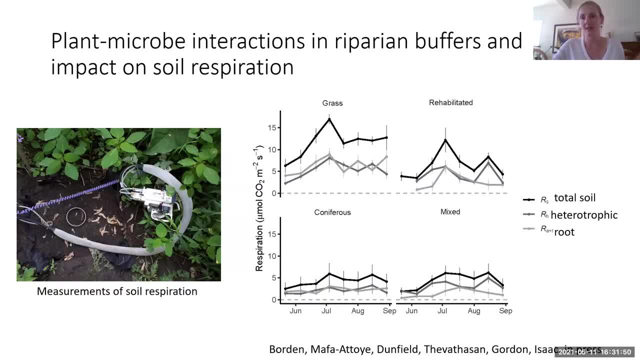 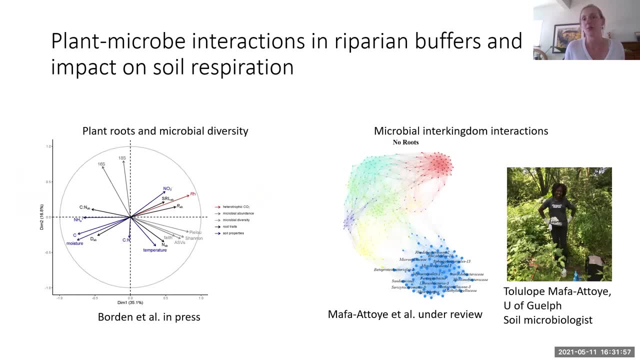 And so we have these, these flux data from different sources, autotrophic versus heterotrophic- and we can relate that to to microbial analysis that was done, as well as other properties like the type of roots that were there, And so I do a lot of functional trait work. 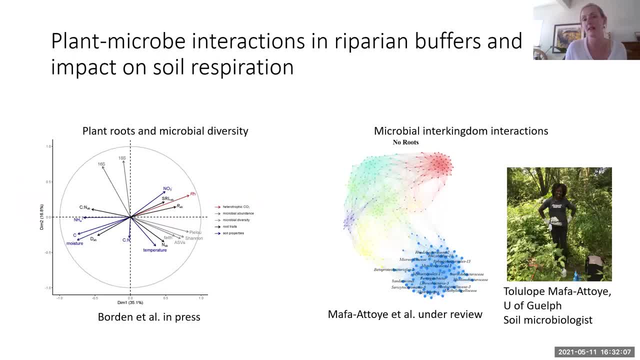 And so I related that to these respiration rates, as well as the soil properties that were there. So I won't go into too much detail on that, but I'm happy to answer questions on that. On the left are some results from the study. 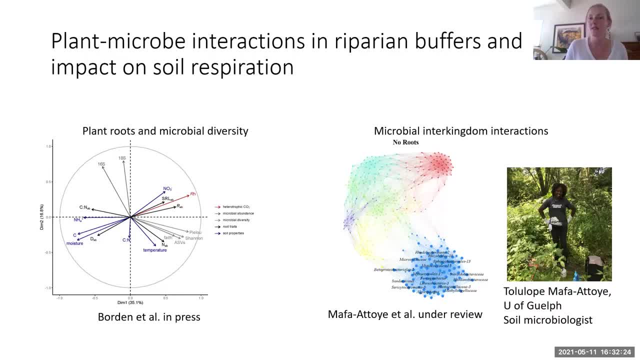 that focused on how to link soil properties with root properties and microbial properties, And we saw these systematic patterns across different types of riparian buffers. And then on the right are some results from a study that's being under review right now. that's led by a soil microbiologist at Guelph. 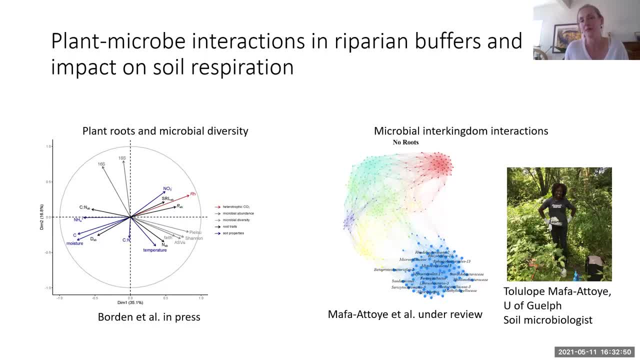 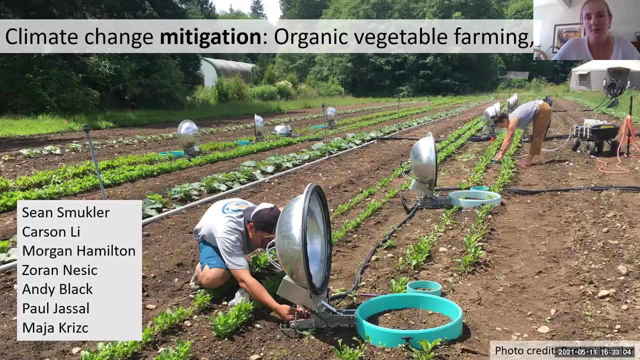 looking at the effects of these root exclusion experiments on inter-kingdom interactions. So your fungi, archaea and bacteria co-occurrences At UBC Farm. this is some work, another collaborative project brought through the Agriculture Greenhouse Gases Program. 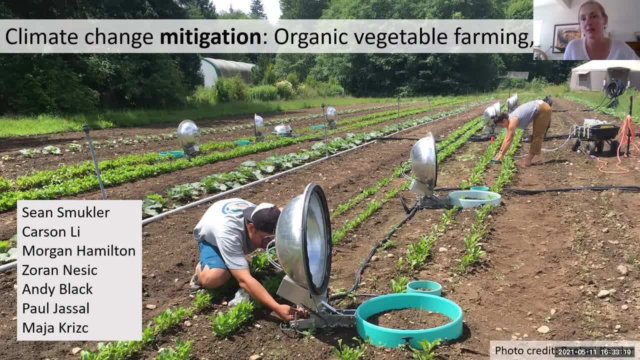 So I can see Andy Block is here, So him and the Biomat group, among others soil scientists, are involved in this work. We can see Carson Lee and Morgan Hamilton working in the field And we've established these auto chambers, So these big domes that close down onto those larger collars. 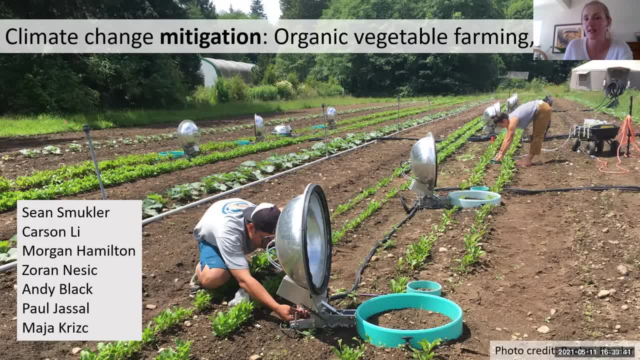 as well as manual collars that are just aside to them And they, you know, as they're closed, they accumulate the greenhouse gases- methane, nitrous oxide and carbon dioxide, and over time, you can plot the rate of emissions based on how they accumulate over time. 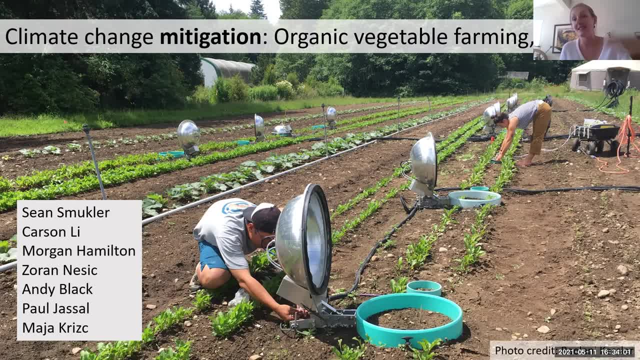 So the auto chambers: they collect the data continuously or kind of continuously throughout the day and the night. And the manual chambers- you know Morgan's out there obviously manually closing a chamber and taking measurements with a gas mat. So we've got a lot of data coming from the site. 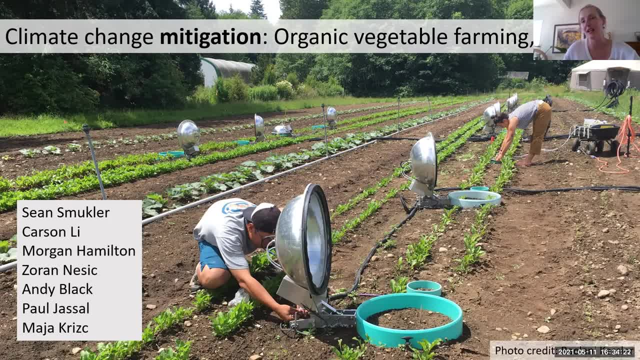 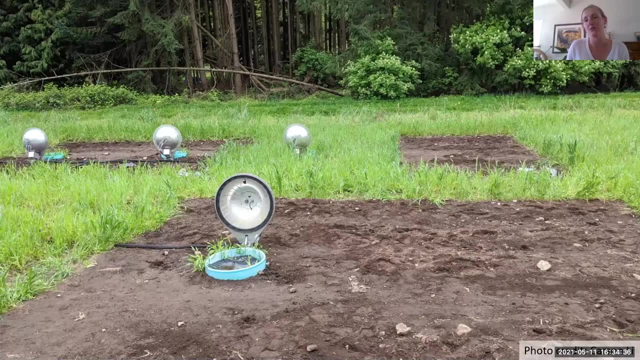 where we've done these treatments of plastic, mulch and cover cropping and different nutrient management strategies, to see how these all interact and how they impact emissions. So again, a ton of data. we're hoping to do some modeling on this, since we have multiple years of data. 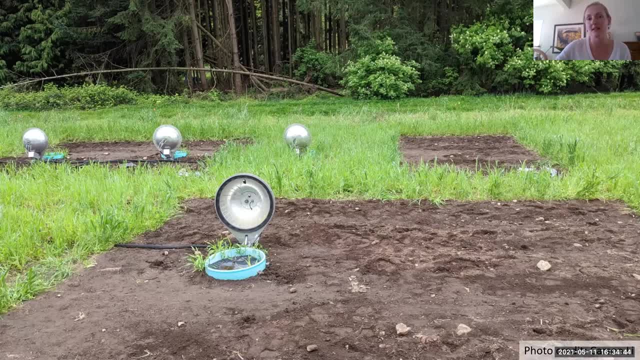 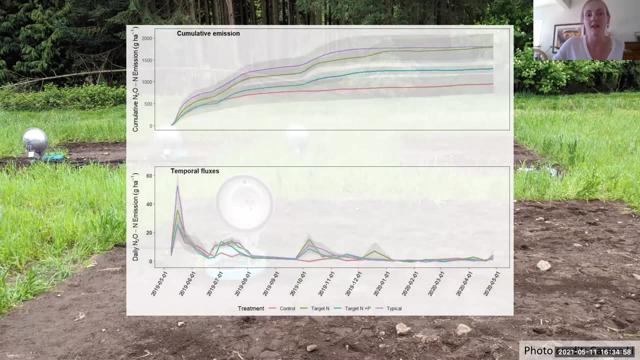 to parameterize some commonly used carbon nitrogen models. Here's some more images of the auto chambers in the field and after the tarps have been removed, and some preliminary data of the greenhouse gas emissions from the following different nutrient management strategies. So on the bottom are these instantaneous fluxes. 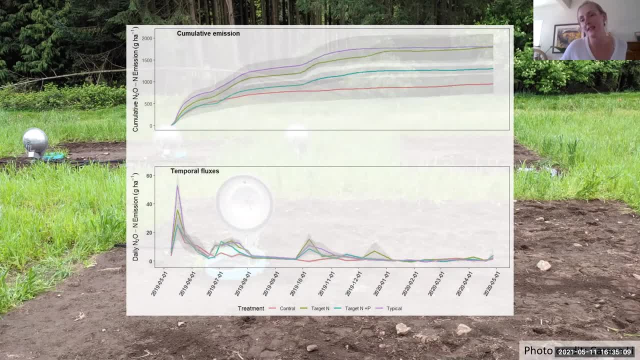 that are occurring and if you add them up over time, we see that treatments were piling on. a lot of compost are emitting cumulatively more nitrous oxide emissions over time. So we're hoping to do some modeling on that as well. And another lovely photo taken by Kirsten Lee: 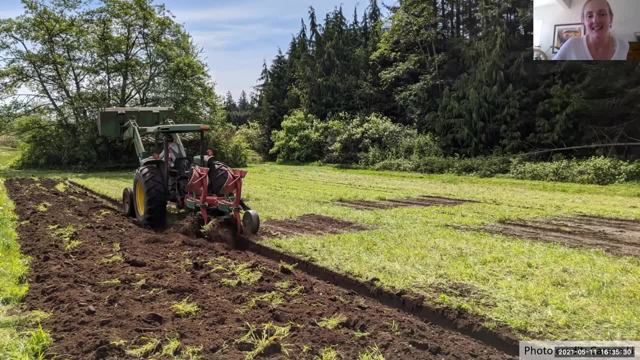 the tech of our group just to go back or, I guess, to think about long-term effects. So we're modifying the soil, not just with what we're amending, but the cover crops that are growing. that's a source of carbon. 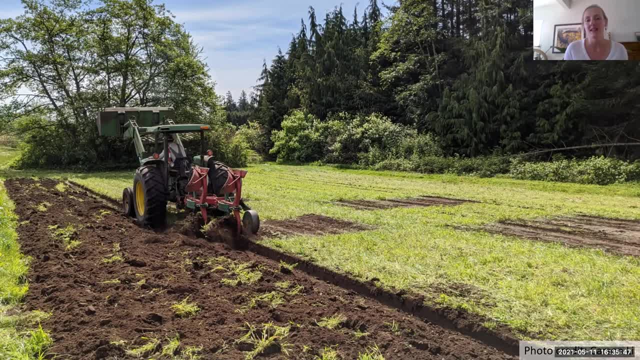 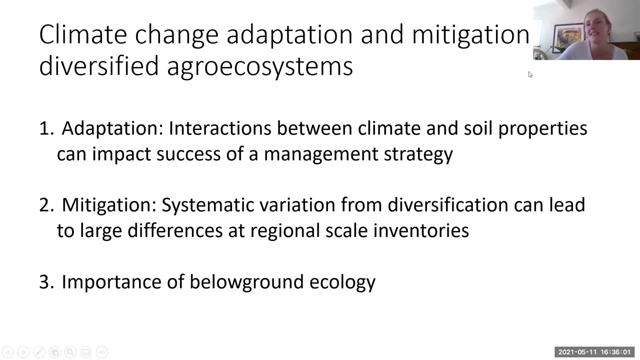 So what happens to that in the long-term? And so I guess just ending on on this beautiful photo of UBC farm is where I want to go. Yeah, so the final, I guess the big three takeaway messages from what I wanted to share today. 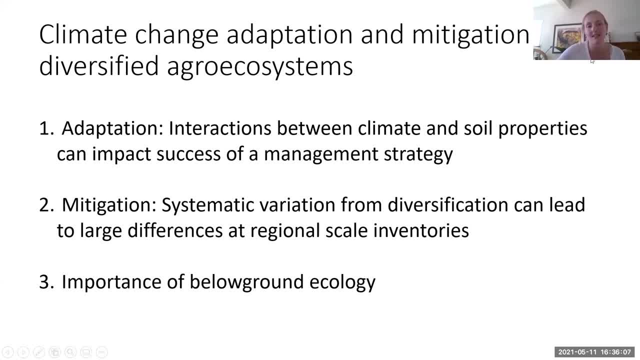 From the adaptation side, the interactions between climate and soil properties can impact the success of a management practice, a diversification practice. From the mitigation side, systematic variation from diversity, diversification can lead to these larger differences for our regional scale and up assessments of. 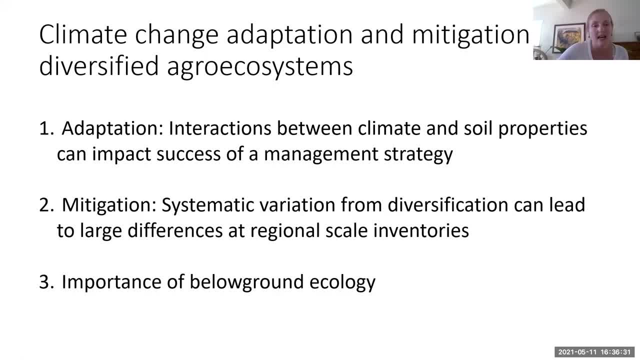 how much carbon is being sequestered or stored, And then, finally, the importance of below ground ecology. So a lot of my work, as you can see, revolves around what's going on below ground, with the roots and the soil, And I work a lot with microbial microbiologists. 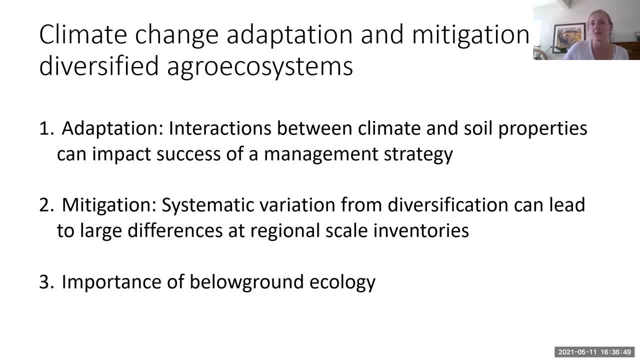 and those are main driving forces of what's occurring. That's driving, you know, driving greenhouse gas emissions from the soil. So yeah, but we don't know a lot because it's very difficult to study and complex. So I think it's exciting times to be involved in this type of 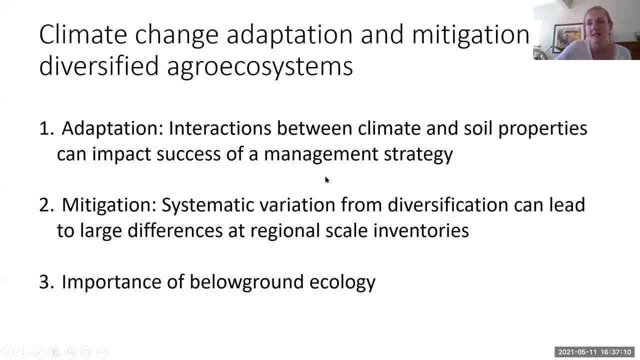 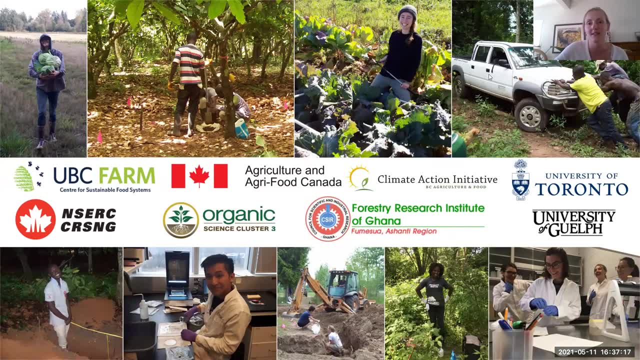 research And with that, just a thank you to everyone that's helped me out in the field and in the lab, and some funding sponsors, of course, along the way. So I'm happy to take some questions and have a discussion, hopefully. Thank you so much, Kira. Yeah, thank you everyone. 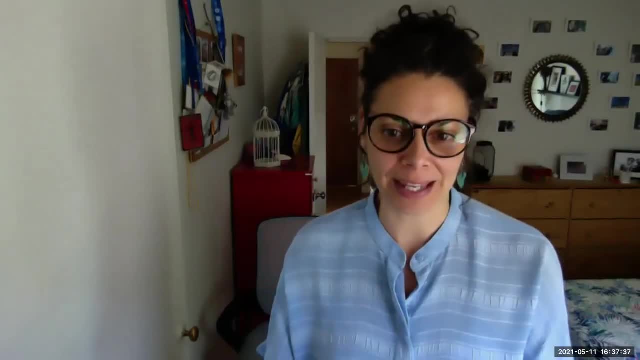 I have a question, but I would like to see if others have questions. So, please, if you want to ask a question, please feel free to ask a question. If you have a question, please feel free to ask a question. If you have a question, please feel free to ask a question. If you have a question, please. 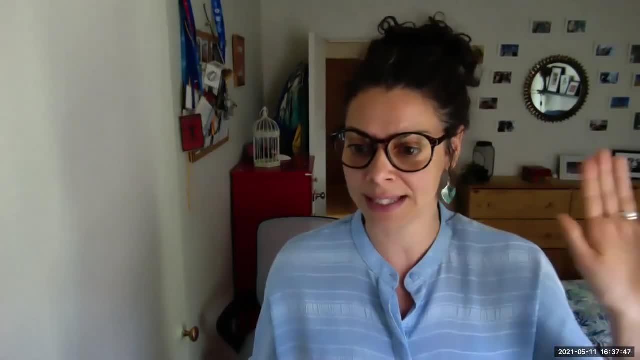 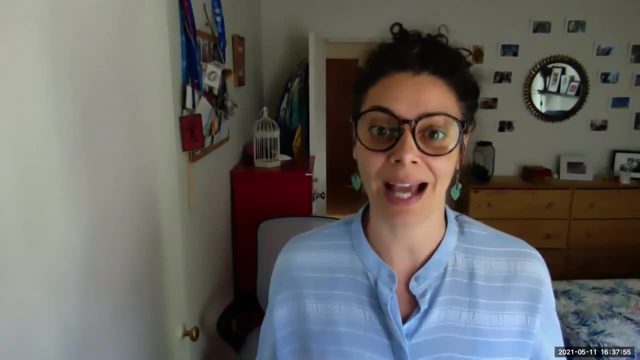 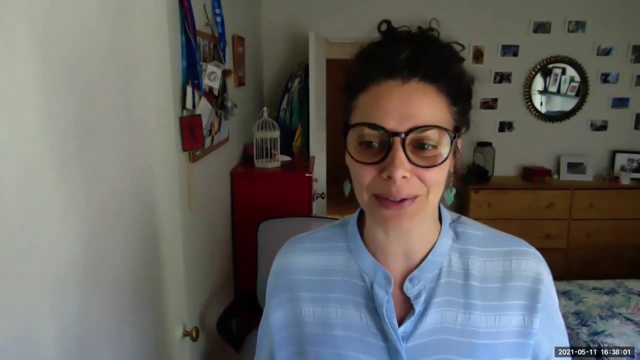 raise your hand And the raising hand. you can find the raise hand button in the reactions section. Okay, Hannah has a question. So, Hannah, I'm gonna ask the first question and then you go, because I'm very curious. You show Kira the cumulative effect of the different. 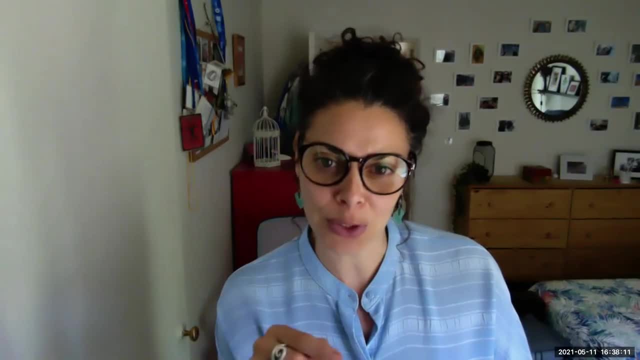 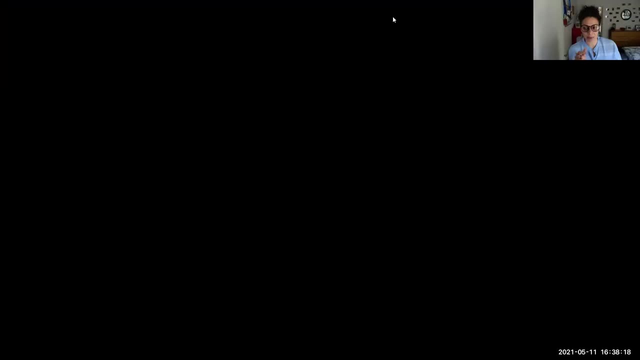 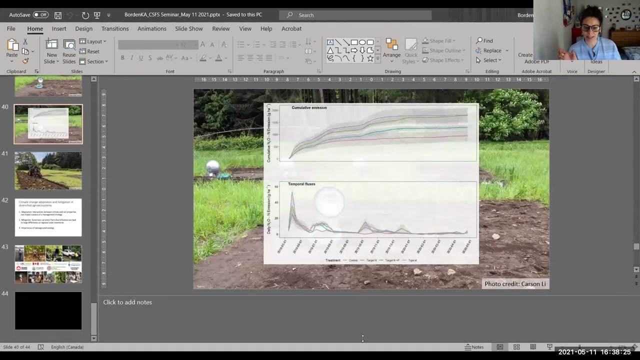 management practices at UBC Farm. Could you share your presentation again- And it was. you didn't describe what the different treatments were, but I saw that there was a huge difference between the typical which- yeah, if you look at the top window. 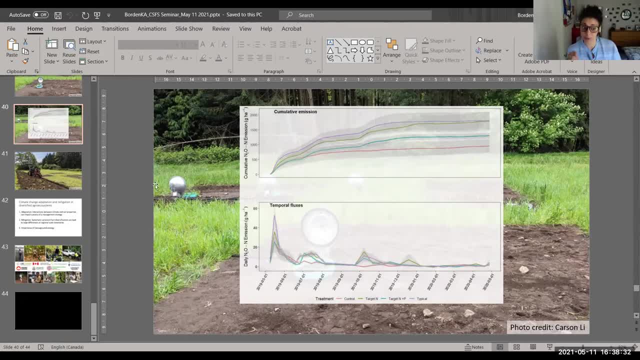 the control is red and it's obviously doing much better in terms of emissions in compared with the typical. So could you explain what was the control and what was the typical management practice that you were talking about? Could you explain what was the control and what was the typical management practice that you were talking about? 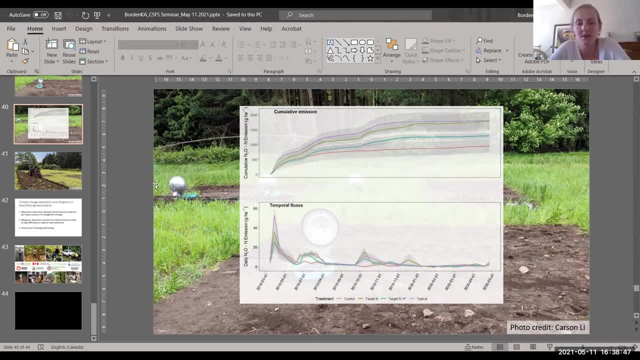 Yes, so control is when we're not applying anything And the typical is what the farm like the farm typical application rate would be. So to measure that, we actually went out with tarps and Tim, or whoever had been managing that plot at the time, would just drive a tractor over and we'd weigh how much compost that they dumped onto. 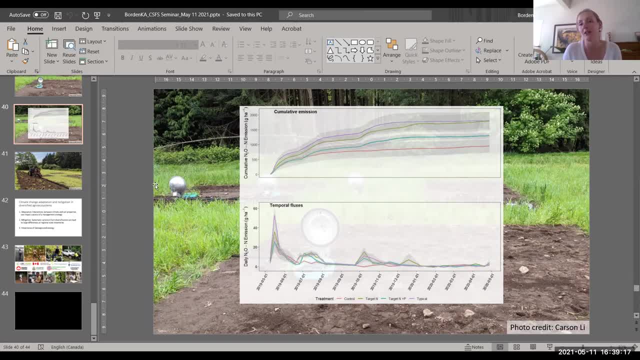 a certain area and we could estimate you know how much compost per area that they're applying And it actually corresponded very closely with our target. N is how we've labeled it here. It's a high compost application, where we're exclusively using compost to meet the nutrient demands of, or the nitrogen demands of crops. And to do so you have to put quite a bit of compost on, Because you know that not all of that nitrogen that you're putting on is going to be available for plants. It has to mineralize first. it takes time, so you put quite a bit of compost. 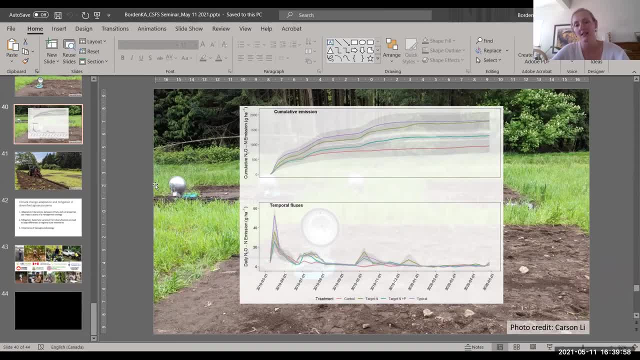 on to do that, to meet the nitrogen demand. So those, the typical and the target N, which are the purple and the green lines at the top, there those are. that's a lot of compost being put on. And if you could go back, or go back in your mind, if I could show you a photo, 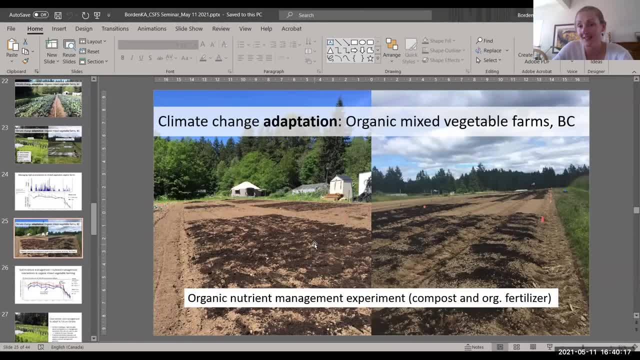 I mean, I want objetos, I want plums, I want, I want- I don't know why are you still here? But that's really what I meant by putting a lot of compost. You know these areas where you see a lot of compost, that's. that's what I mean by. 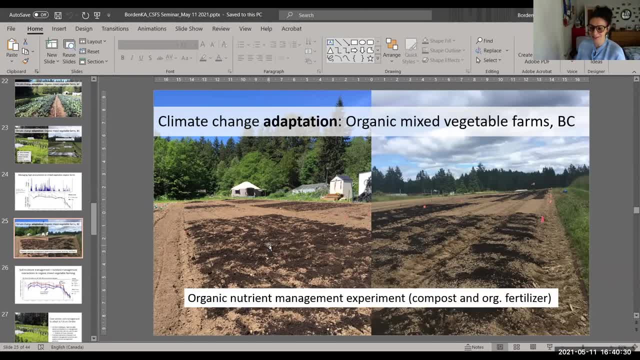 quite a bit of compost being put on. MK H Sparky. Yeah, Thank you so much. I was curious And Okay, so, Hana, you go next. You can unmute yourself and ask your question. HANA, HA大家都選ettu Veronica. Great thanks, Kira. I'm not sure how I missed the vote that you're. 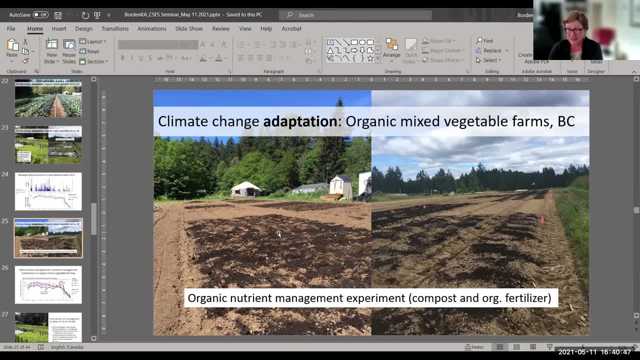 a huge body of work and very impressive. I have a couple kind of two unrelated questions, but coming from the side of kind of farmer driven research and then also thinking about the applicability of some of this to farmers, real lives, and one of the things that we're finding a lot is that 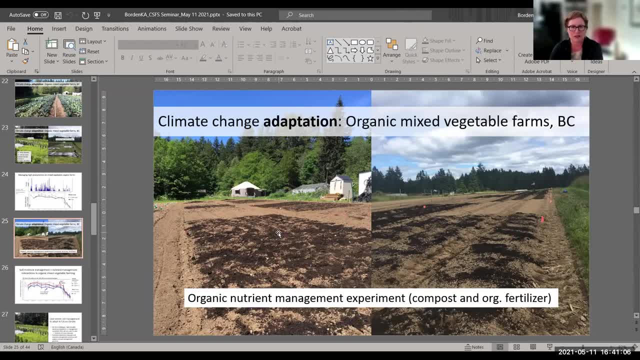 diversification brings a lot of social and economic challenges, like there's the, because of its labor intensiveness, because of the additional layers of knowledge that are needed. you know, the more crops that you're managing and the more you're you're kind of mixing them up in different 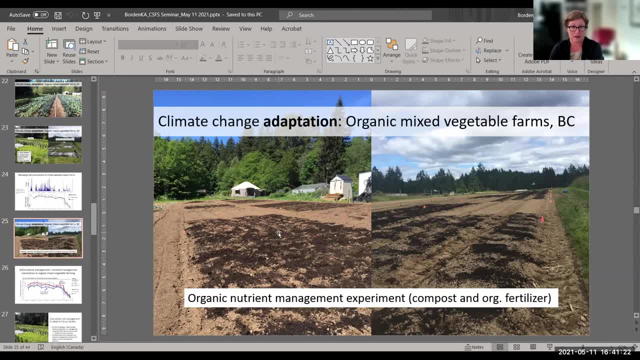 ways. there's different kinds of knowledge that are needed and it's just a more intense system. So I guess my first question- then I'll ask the second one, maybe after everyone else has had a chance to go- is: to what extent are you guys studying the labor implications of diversification? 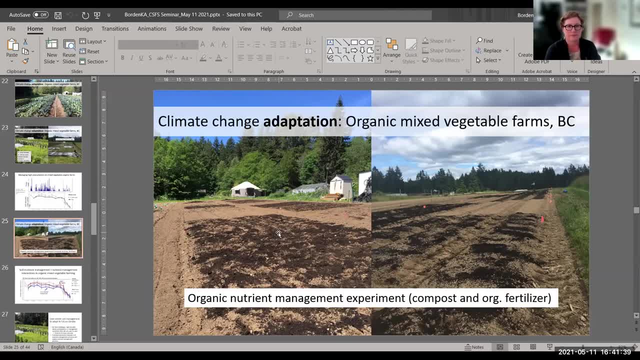 and kind of including that in your cost-benefit. Yeah, so that is getting. that's an excellent question and that is getting included in the analysis for UBC farm work, since we have the cost of the, the inputs. so that's one indicator of you know. 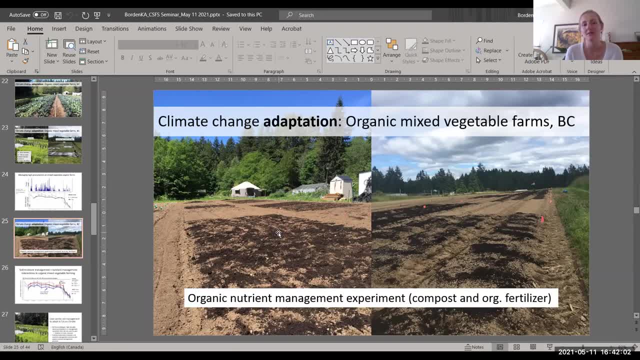 the, I guess, the economic input in terms of, like the physical, but not just the inputs themselves, with the labor to apply them and harvest And manage and all that kind of labor. So I guess, in terms of if you were to relate labor, of comparing a monoculture versus a mixture of crops, that's- yeah, that's definitely not part of 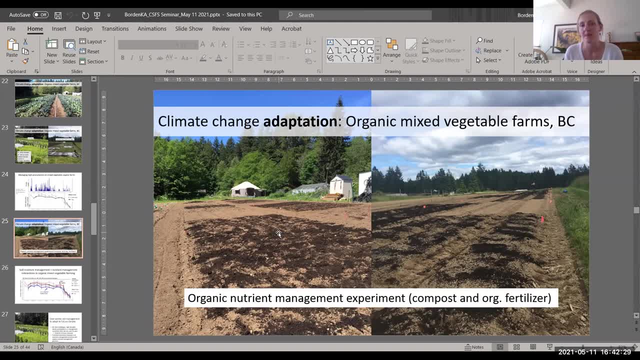 the data that we'd be collecting. That would be very interesting to have that kind of gradient of diversification and see the labor requirements along that gradient. but these are all about. I think I saw Amy Norgard on here, she did the regional analysis and and Rilani Kessler is doing 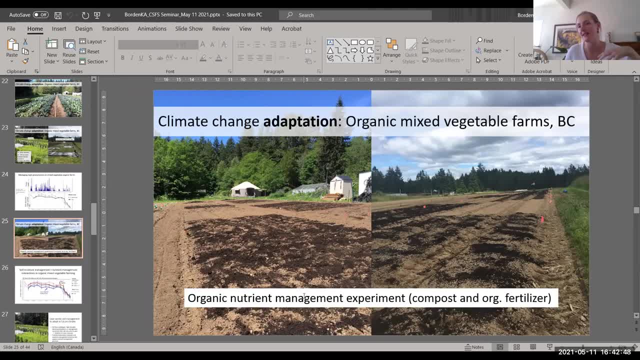 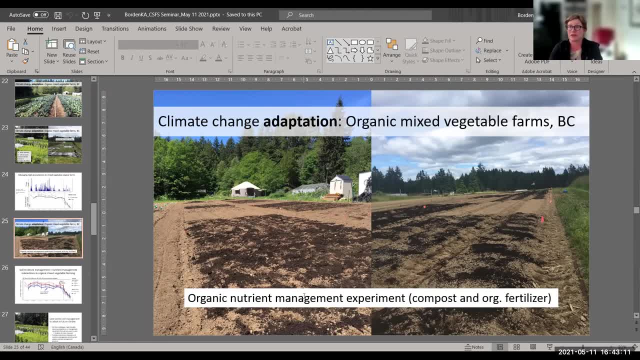 Yeah, I think they are trying to track it at UBC farm, But I guess it's more a bigger question. just from your, your research and these other contexts as well, to what extent did farmers talk about the labor, labor being a constraint or not to diversification? 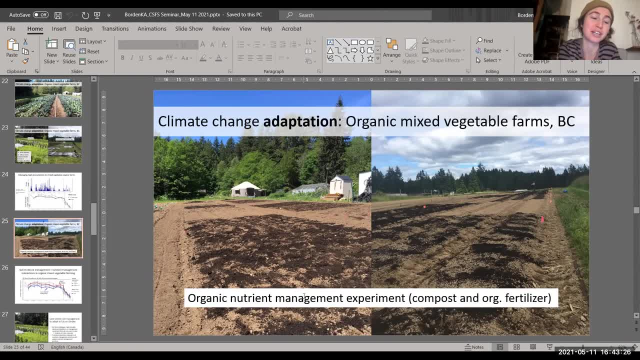 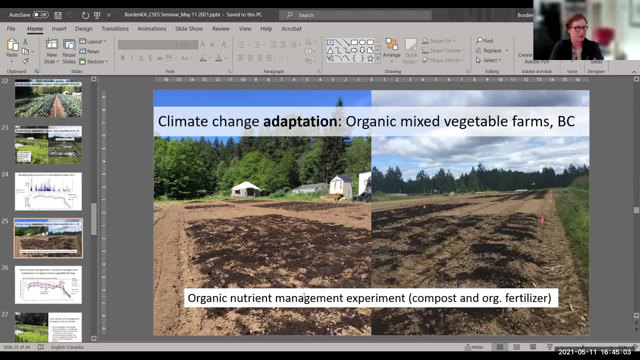 And then I just on that last point, you talked about the future directions and the blow ground ecology, which I find fascinating. And again, looking from a farmer perspective, are there ways for farmers to get involved in more self-assessment of soil health? 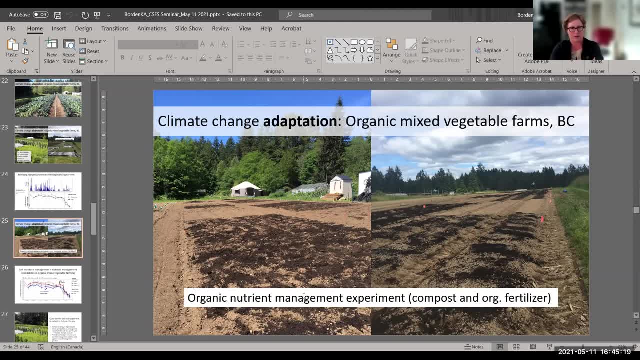 And I was just curious kind of any ideas you have about, you know, especially farmers who may have fewer economic resources- you know they can't run around sending soil samples to the lab all the time- And what are some ways that you've found that farmers can kind of self-assess soil health in a way, that kind of maps onto or approximates the kind of estimates that you're able to get with these like amazing pieces of equipment? 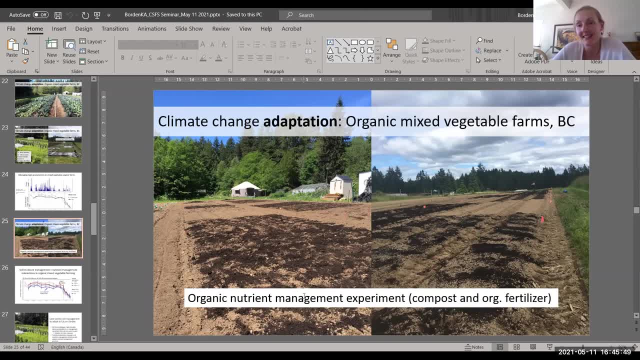 Yeah, So I suppose an easy one that farmers would identify already in cocoa systems is mycorrhizal association. So cocoa do form mycorrhizal associations and you can see it. It's a very visual indicator. It's a very visual indicator of that process happening. 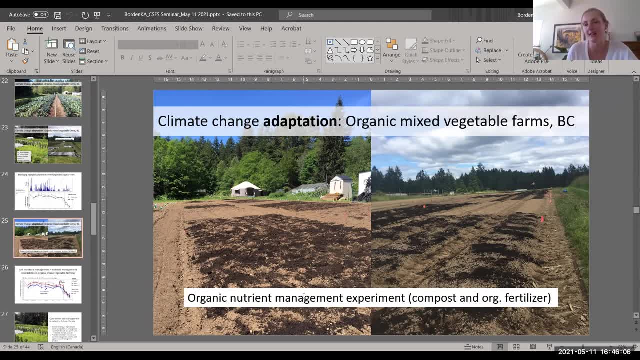 And you know there's some work looking at, you know, are there more associations in monoculture versus more diversified systems or the other way around? And yeah, so that's one kind of visual, easy indicator that a farmer could use without having to send soil samples away. But yeah, I mean, that being said, Just for perennial crops, or would that work for annual crops? Yeah, you could use it for annual crops. I mean the brassica. it depends on the crop. Brassicas generally don't form mycorrhizal associations. 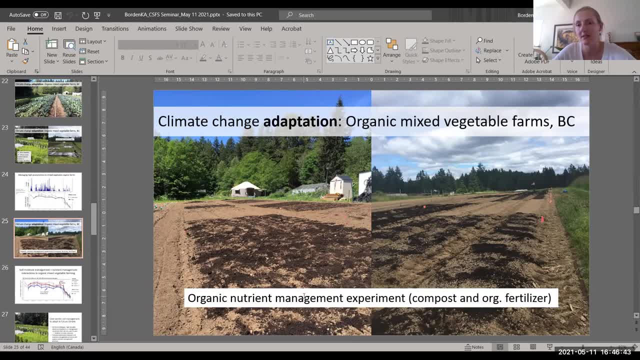 Others are more, might have that, Like a grass type of species or forages might show that type of process happening. That being said, you know analyzing soil, Or the DNA profiles of microbes and soils, becoming increasingly more accessible, so it could become something more accessible for other farmers too. 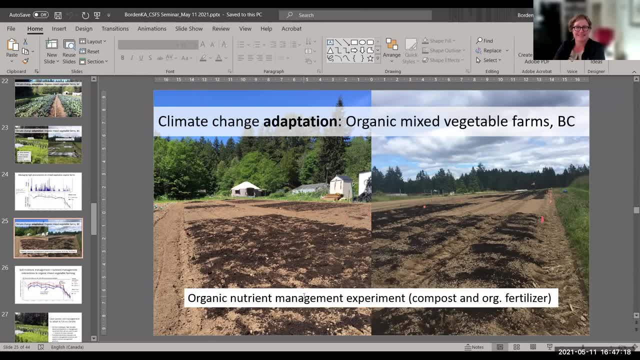 Cool, Thanks, Yeah, thank you so much, Hanna. I don't know like is anyone else thinking of any questions And they are being shy. They are being shy, I just want to, okay, Amy. Amy has a question. 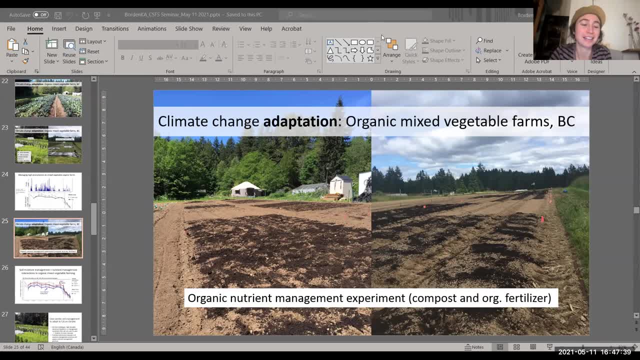 Amy, go ahead. Great, Great presentation, Kira. It's really interesting to see- like the vegetable, I guess- research in the same presentation as like the cocoa. My question is for the same graph that Laura was looking at earlier: the GHG emissions from the different treatments. 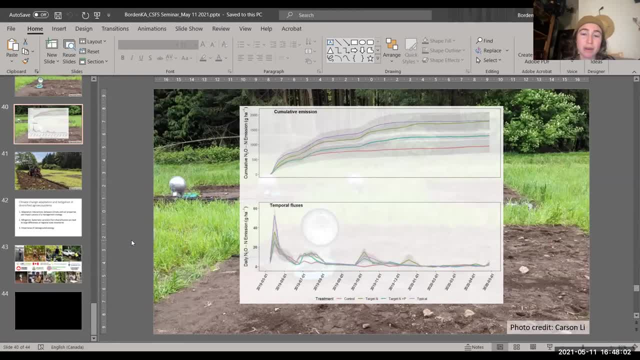 So it kind of seems like you're looking at the same graph, So it seems like you're finding. basically what Gabriel was finding as well is like we have these high N2O emissions from like high compost or manure applications. 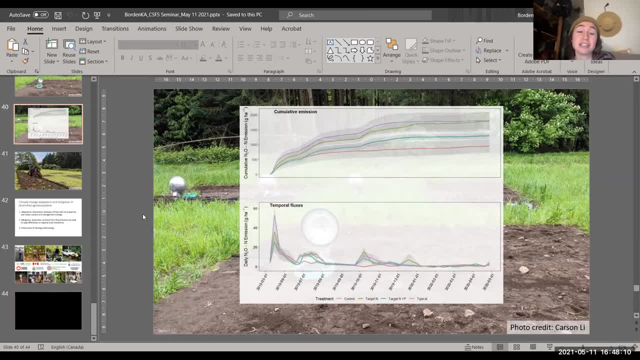 But then I also feel like he was finding like a yield tradeoff with that. I'm not too sure if you've looked at your yield data yet, but is it following kind of like Gabriel's pattern of so like you're having the high N2O emissions from those treatments but those treatments are also yielding slightly higher than the other ones? 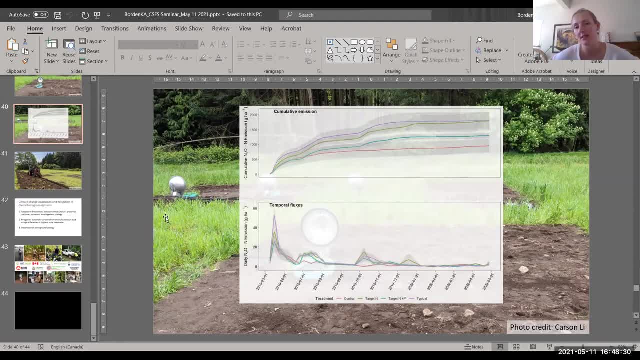 Yeah, I think you may have seen some of the yield. Yeah, I think you may have seen some of the yield data at one of the conferences we've presented at. But yeah, there are no differences among the different treatments, So there's more yield than when you're not applying anything. no surprise. 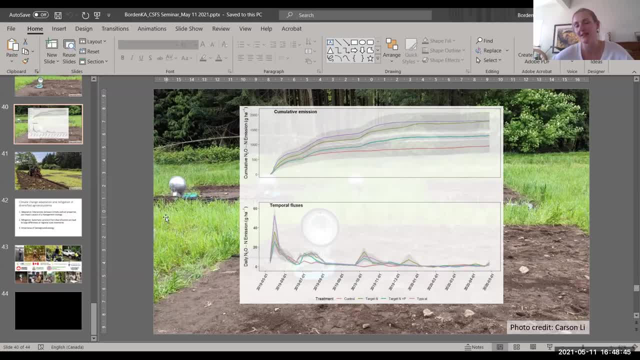 But so yeah, there's no. from the initial data set that I've worked with so far, we haven't seen that type of tradeoff in yield output among the different strategies yet. Sweet Yeah, I feel like that's what I remembered seeing. 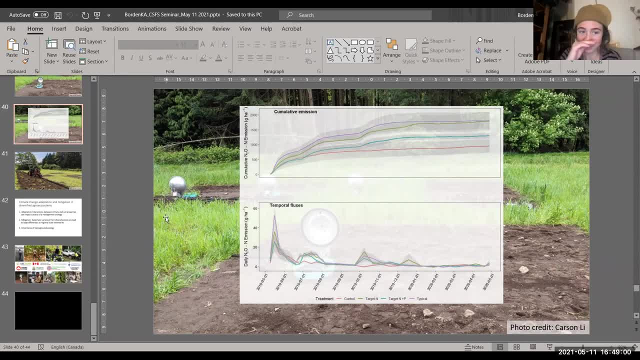 I just wasn't too sure if those were like super preliminary Or if that was starting to be a more complete data set. But it sounds like you're still. Yeah, I haven't looked too in-depth at where they've tracked from last summer. 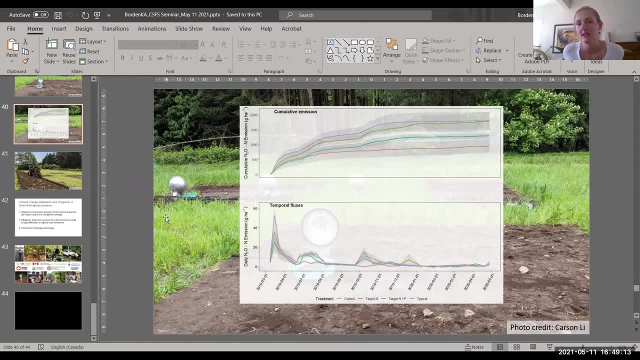 I haven't looked at that data set yet. Sweet Thank you. Oh, Andy Black is just like very happy with the results. Yeah, so, Andy, do you have any particular questions? Yes, There you go, Andy. 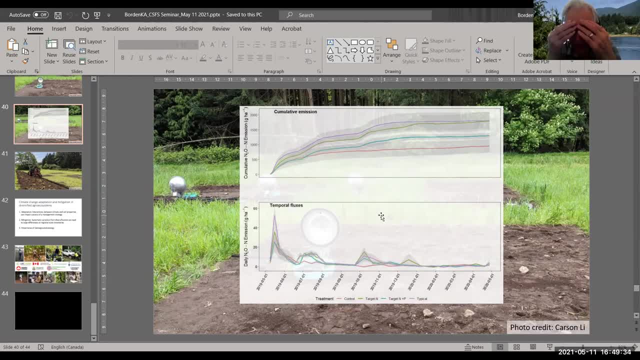 Go ahead. Yeah, I have a question. Yeah, it's very interesting to look at the cocoa shade system And I was wondering how old is a plantation like that? Is it 20 years old? I don't have any idea. 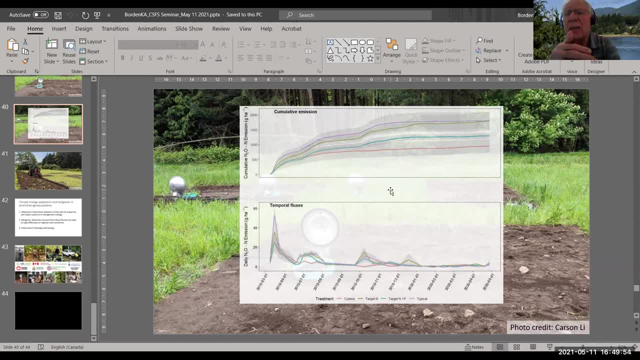 And does everything get planted at the same time? I mean, what I'm getting at here is the amount of carbon that you see in that stand, Like the above ground That's accumulated over the life of the plantation right. So divide your numbers by age and you have a rough approximation of the rate of carbon sequestration. 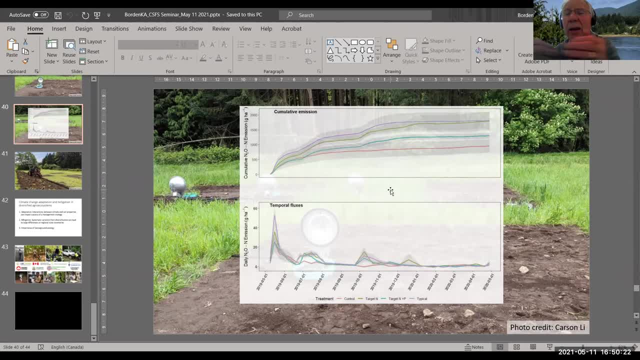 Right In tons of carbon per hectare per year, And I was just wondering if you thought about that. I mean, I'm also interested in Mm-hmm, Mm-hmm, Mm-hmm, Mm-hmm. 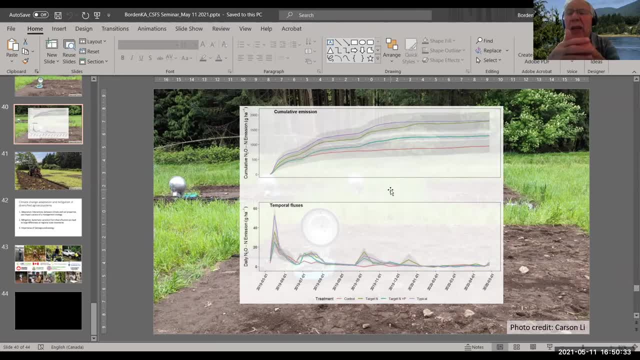 Mm-hmm. So what's happening in the soil in terms of carbon? Is it declining? You accumulate in the above ground. What's happening in the soil? do you think Yeah, so for the age of the plantations? cocoa starts producing cocoa pods around five years into their lifespan. And then the varieties that are commonly Like the main ones that are relied on in Ghana, probably a 20, 25 year lifespan. Some other varieties do go for a lot longer. They'll go for 50 years, which is pretty neat. But yeah, there's certainly. I mean, it's a bit of a- I don't know if I want to say can of worms, but it feels like a can of worms when we start talking about carbon storage temporally in forest systems. 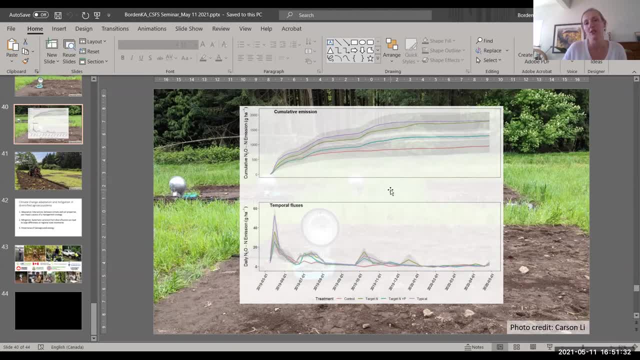 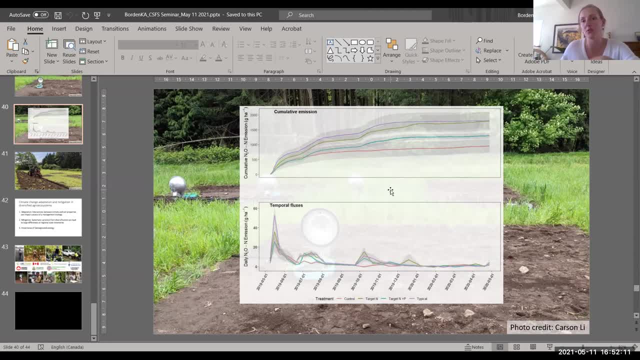 if it's a shade tree might already be there and cocoa get planted underneath. So that would be the other pathway. Some of our forest systems. here we'll see lots of carbon sequestration. above ground right, Big trees are growing, but in the soil we'll even see 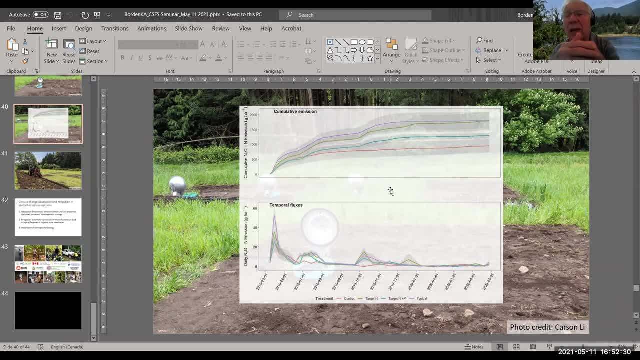 declines in the, in the amount of carbon there. So you really you're paying a high price for that, for that accumulation above ground that eventually goes off to the mill or wherever. wherever it goes, Yeah, Yeah, There's certainly. I mean it's very complex because even the shade 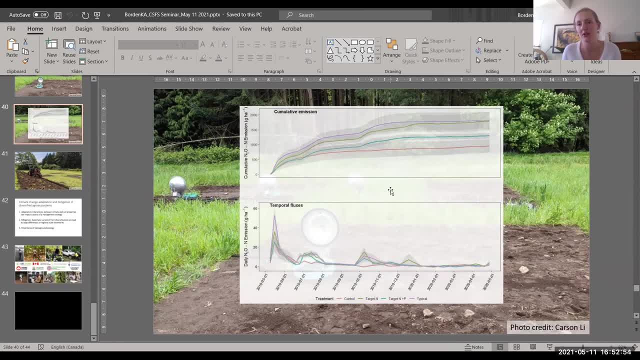 trees, they're going to have different litter types And so they're going to drive different types of nutrient cycling In the soil. But yeah, these are. these are all questions that get asked in much of the research of agroforestry- cocoa agroforestry and related to carbon. And then there's lots of context. 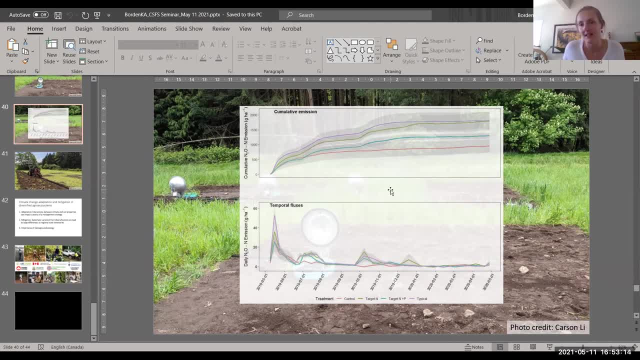 specific results that say yes, there's more carbon and some no. there's no gains in carbon in the soil with agroforestry, It depends. Yeah, Yeah, Thanks, Thanks, Kira, That's good. Yeah, I have a follow up question, Kira, about that. And and in the meantime, if anyone has, 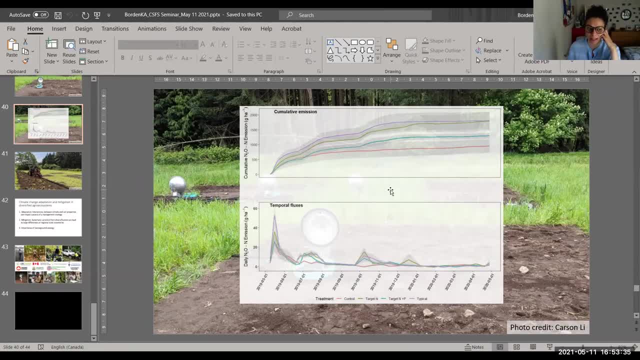 an additional question. please raise your hand and I will. I will allow you to ask the question. but yeah, about the cocoa. So you basically were looking at three factors, right, Like growing, growing cocoa by itself, without the agroforestry, kind of like the, the diversified model, and then 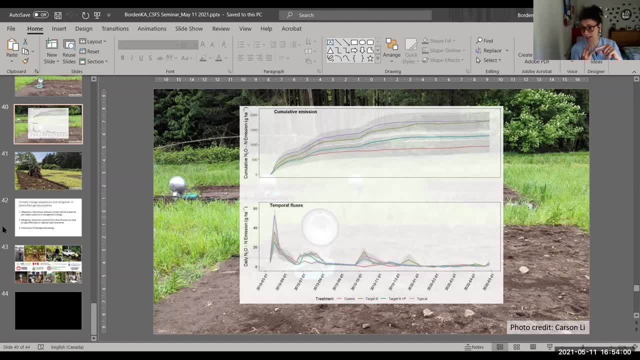 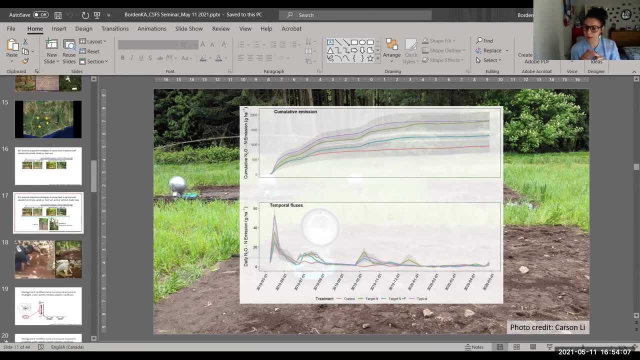 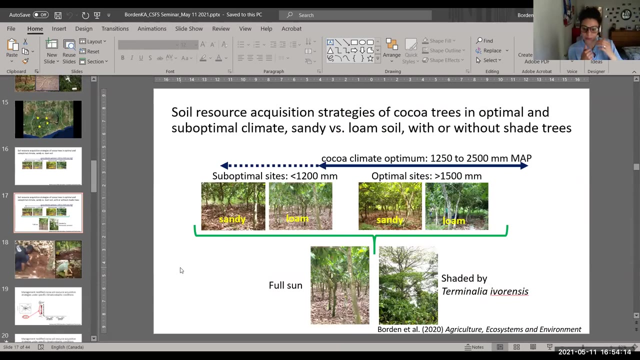 that was shaded or not shaded. right, That was the factor. And then you also had a type of soil And what else do? I think you had like three different things that you were looking at, And, and I just want to, yeah, yeah, there you go, So, and and then you also had like two. 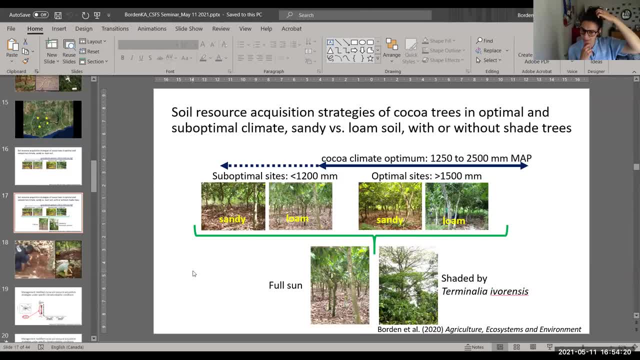 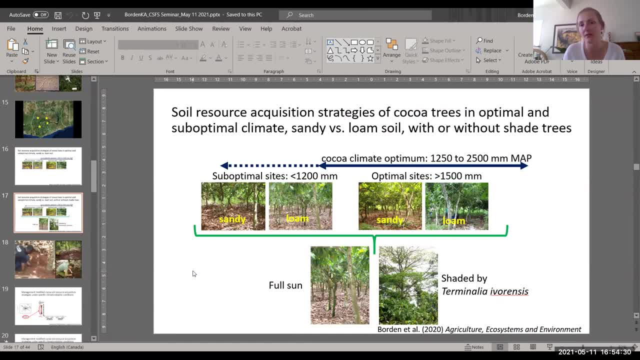 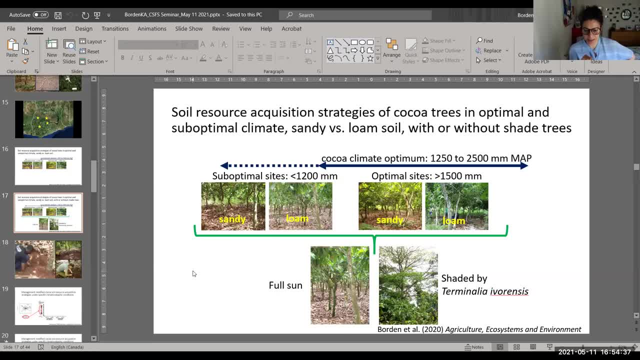 I was curious, like I think it's a few slides after that- Basically, what was the system that was working better, And particularly in the suboptimal sites you mentioned that you were looking at like, like very great conditions to grow this, this agroforestry system. but then 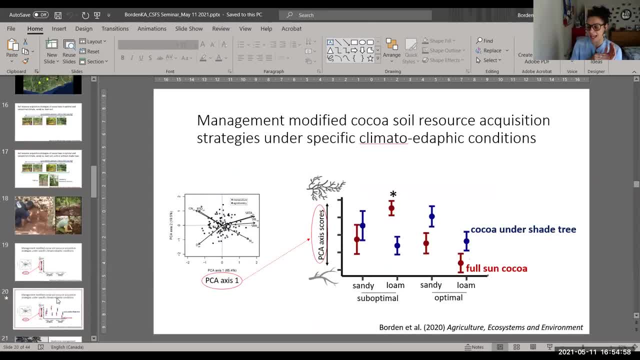 going into the suboptimal sites you mentioned that you were looking at, like like very great conditions to grow this, this agroforestry system, but then going into the suboptimal sites, like closer to the savannah. I'm curious about that kind of analysis I imagine you look at. 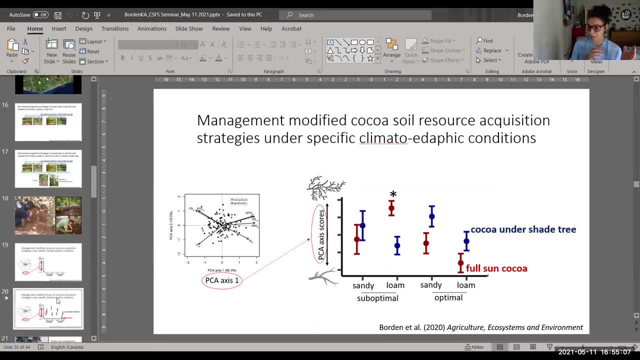 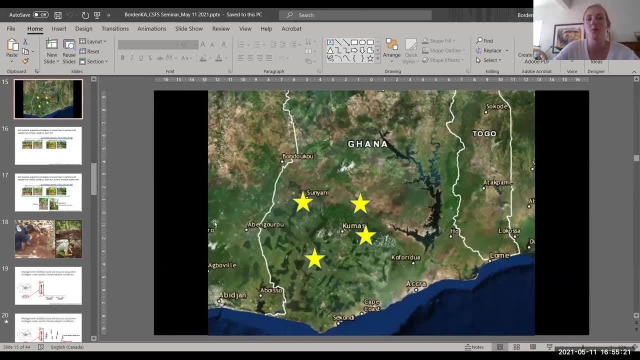 these suboptimal locations as a way of mimicking, like potential climate change conditions. Am I right? Yeah, I guess I should have said that. Yeah, So the climate gradient: we've got these suboptimal locations and more. I think it's nearly half of what's currently. 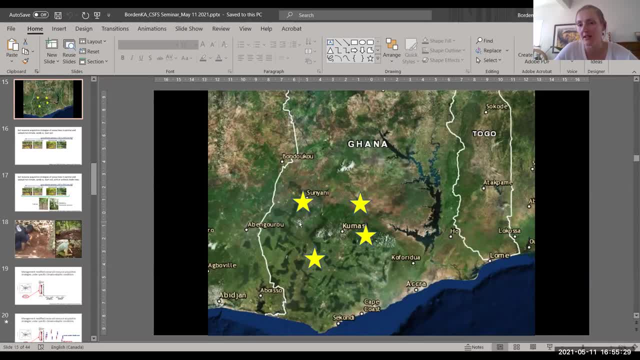 optimal. So we've got these suboptimal locations and more. I think it's nearly half of what's optimal. So we've got these suboptimal locations and more. I think it's nearly half of what's optimal is going to shift into the suboptimal category of cocoa cultivation in the next few. 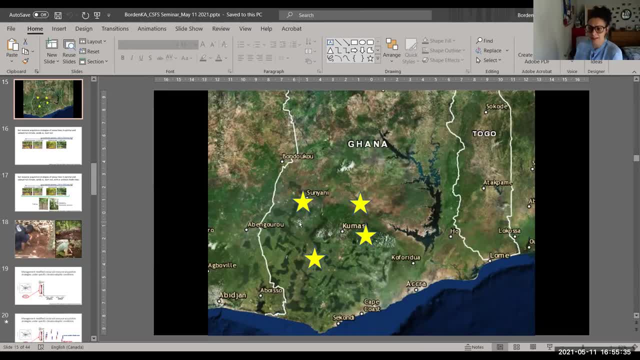 decades. And what was the system that worked better, based on your analysis, in that, in those suboptimal conditions to grow cocoa. So I don't want to say which works better, but that we identified sort of a way to first use some sort of repeatable measurable. 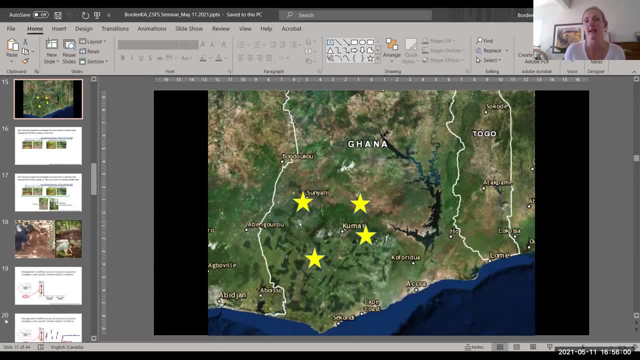 attribute, So these functional traits that we're measuring as a way to indicate what's happening more systematically across these different gradients: soil, climate and species diversification. Of course you'd want to know what yields the response, the yield responses, But that data is. very difficult to get. I won't go into the challenges on that, but there's trade-offs So maybe you don't want to grow something that's very fast growing in a drier condition. I know farmers prefer to have maybe fruit-bearing trees so that they can diversify their income and food. 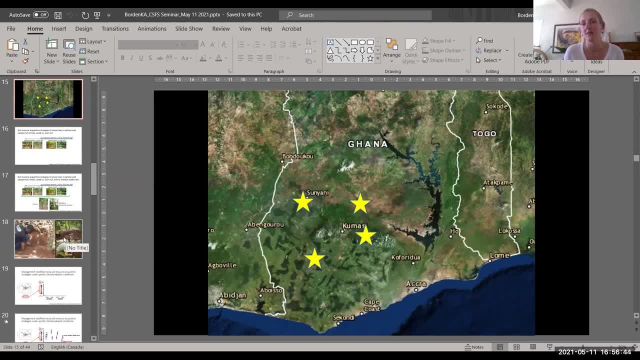 sources in more drier conditions, Whereas in more optimal conditions a farmer could implement these fast-growing carbon sequestering trees more readily. So there's some, I guess, different decision-making that would go into that. So I don't want to go into the challenges on that. but 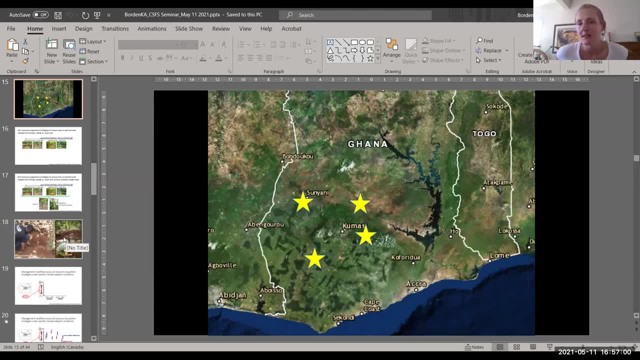 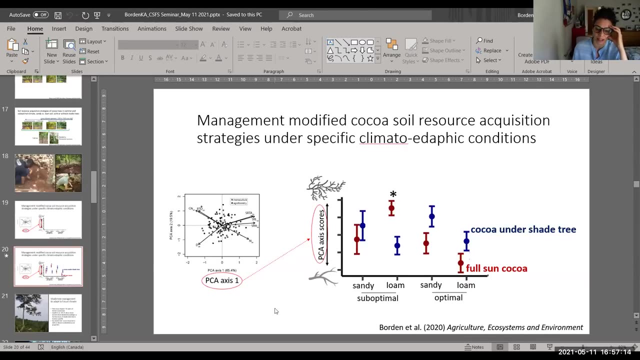 there's a lot of work involved that would get implemented. Does that answer your question? Yeah, I'm trying to connect your previous slide where you showed the different results from those different factors. Yeah, that one I'm trying to, Which is better? 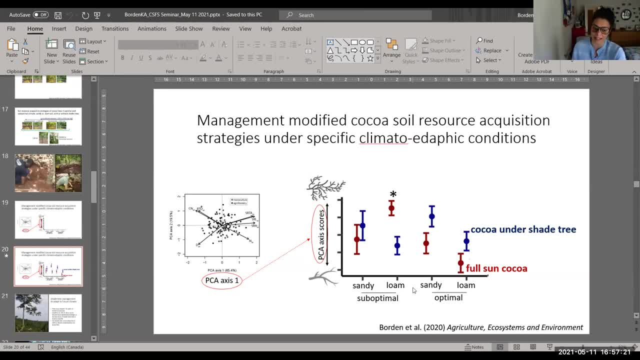 Yeah, Is this in any way answering In terms of- at least in terms of- carbon sequestration? yeah, I'm a little bit puzzled with this figure because it passed by fast and I'm just trying to understand this figure a little bit better. What was your learning from this figure? 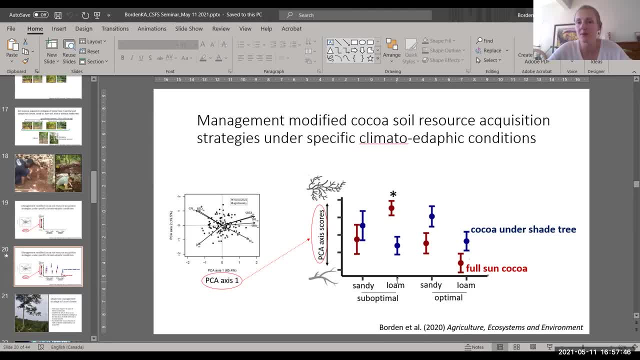 That is under certain conditions that this particular shade tree actually has an effect on cocoa nutrient acquisition strategies or soil resource acquisition strategies, And so it could impact for negative or worse what that is. That requires a little bit more of a specific long-term study, but it's kind of identifying that it's only under certain. 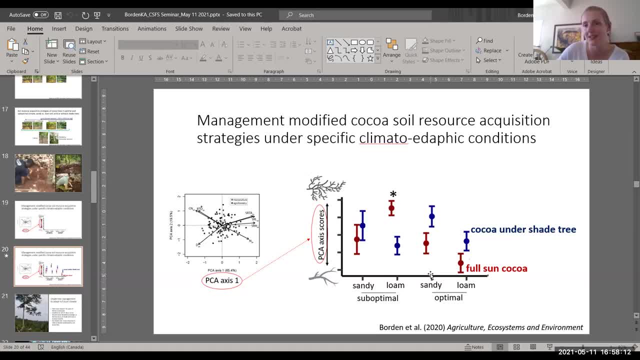 conditions that it has that type of impact, And this particular fast-growing shade tree species does that. Yeah, yeah, I think I understand this now better. Okay, yeah, it sounds very interesting and such a different systems. Yeah, yeah, I think I understand this now better. Okay, yeah, it sounds very interesting and such a different systems. 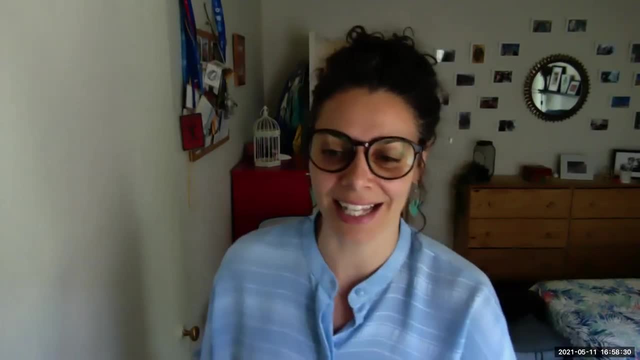 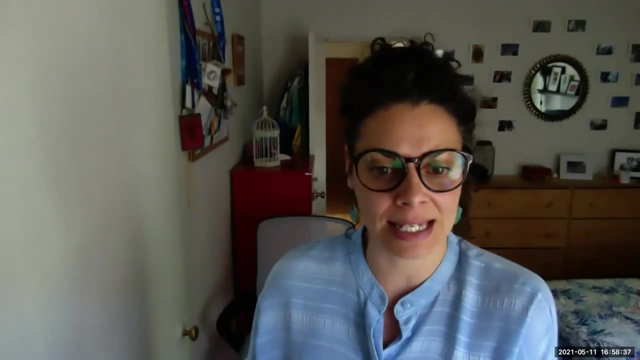 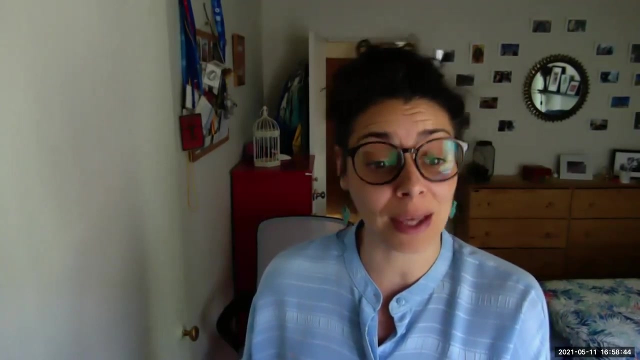 that you have been working on Ghana and Vancouver. it's amazing. So well, I think. if no one else has any additional questions- And I see people are already thanking you- I think we can wrap up. Thank you so much, Kira. It was wonderful to have you. 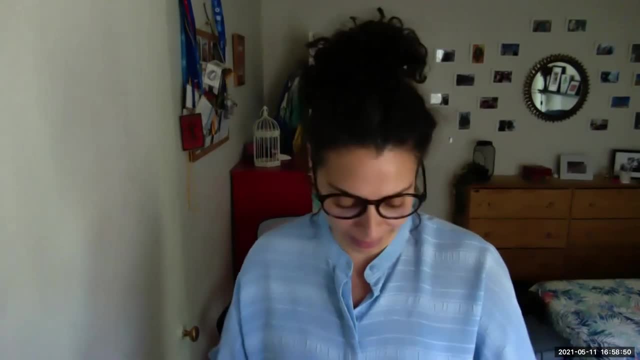 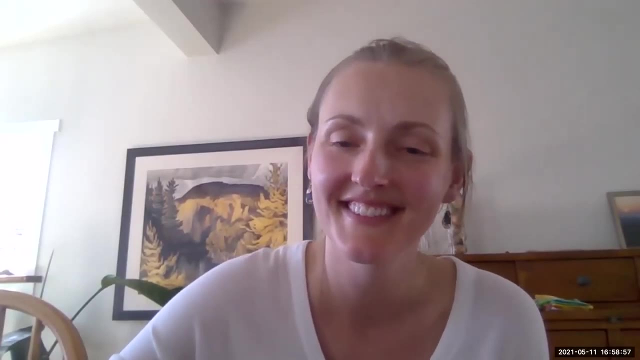 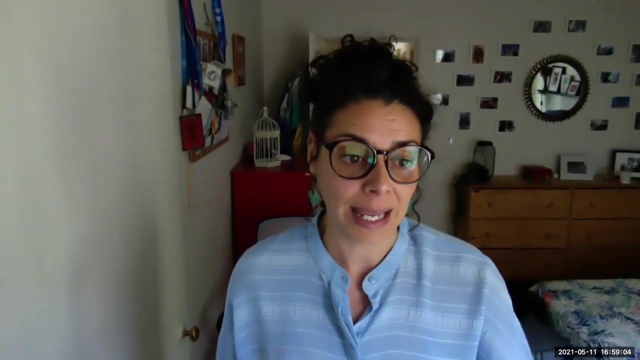 back. I know you have been busy with other more like life-important things like growing a baby, So congratulations on that as well. So thank you so much for bringing these results and this body of research- And yeah- behind the scenes. 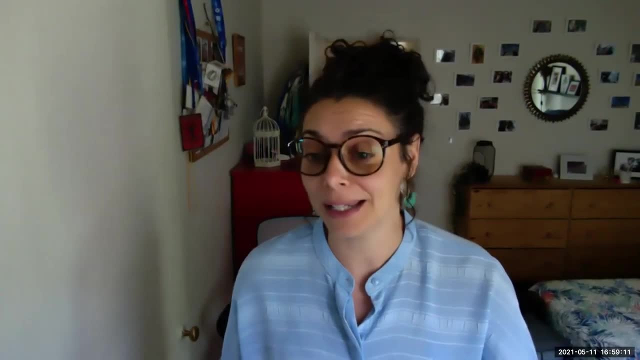 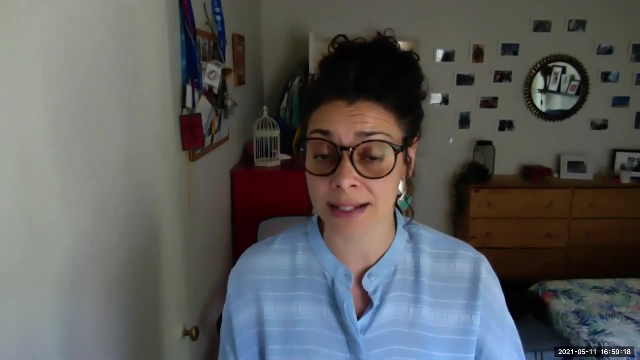 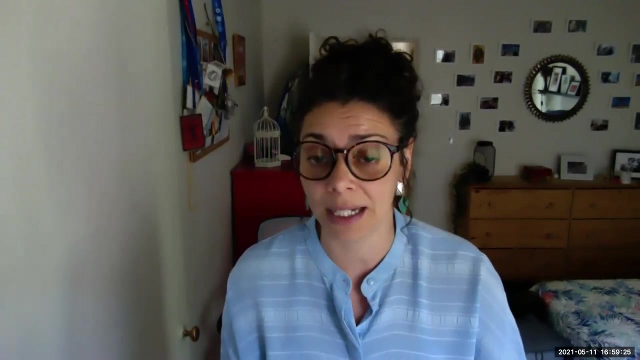 I would like to also thank Melanie Kuchner that was helping me with the technical details, And please join us for our next CSFS Associates seminar. that will be on June 14th, And we will have Dr Simone Castellarín telling us about his research in wine and berries.